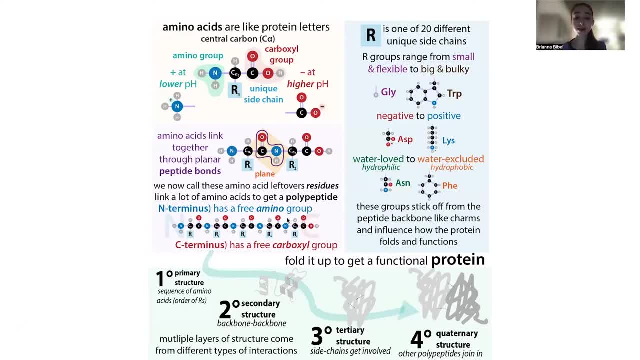 peptide bonds to form long polypeptides that fold up to make proteins. But, unlike the other amino acids, threonine has a unique side chain. Well, they all have unique side chains. These unique side chains, or these R groups, are the parts that stick off from the backbone. 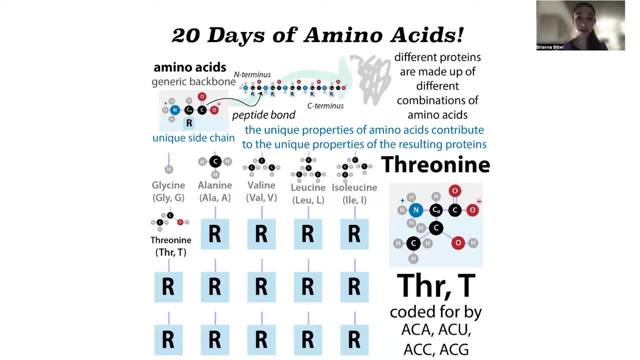 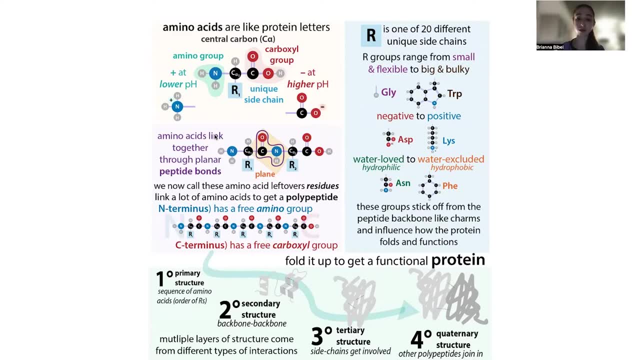 kind of like charms in a charm bracelet. Different amino acids have different shapes and properties, things like differences in charge and size, whether they like to hang out with water or not. Threonine is therefore going to fold up in a way to accommodate all of the different preferences. 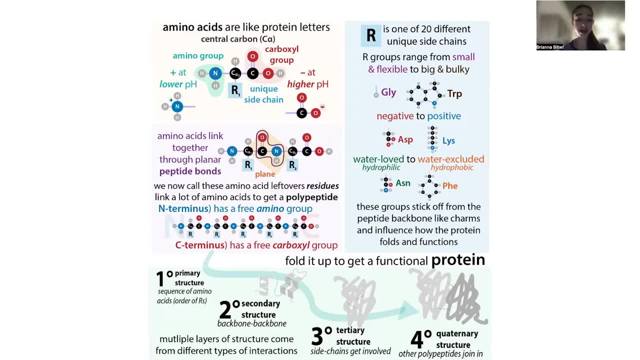 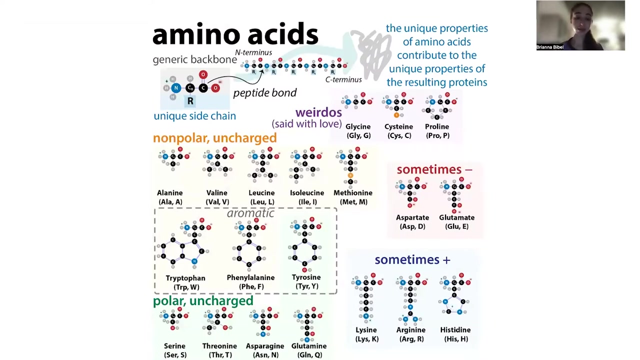 of those amino acids, And because different proteins have different sequences of amino acids, the different proteins are going to fold up differently and make functional products that do different things. What those different things are is going to be dictated in large part by what properties that side chain, what properties that R group has, And so we can broadly classify. 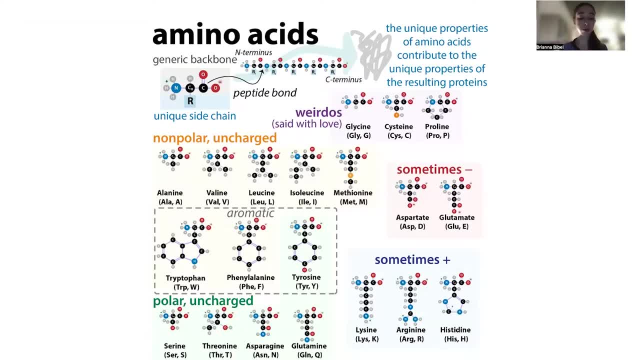 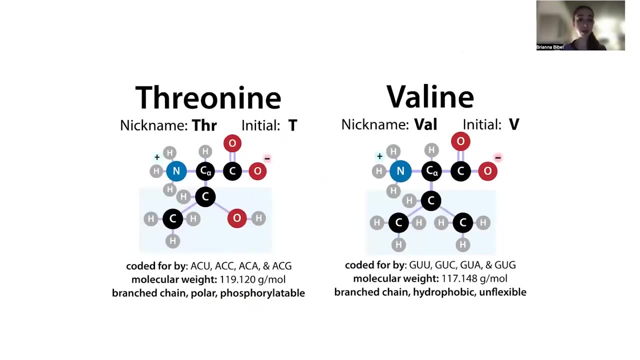 them as like being nonpolar or being polar, And this refers to whether or not they have a separation of charge, And this matters because water likes to hang out with charged things. So if you look at threonine, well, it looks a lot like an amino acid we looked at before phthalene. They both have. 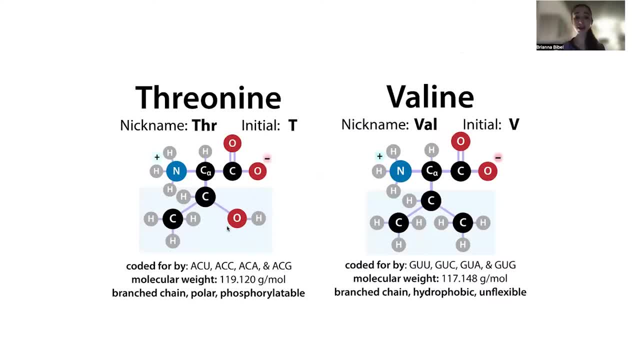 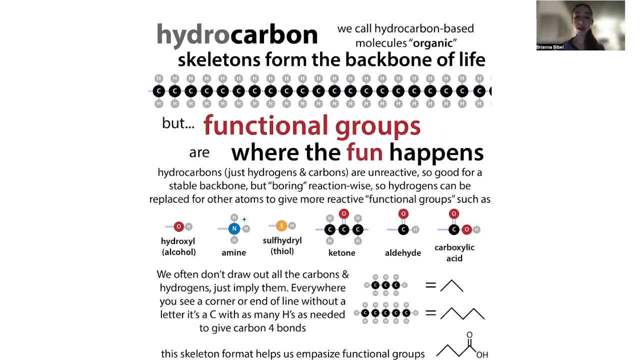 a similar kind of B structure, But in the case of threonine we swapped a hydroxyl or an OH group, Also called like an alcohol group, for a methyl or CH3 group. Now this might not seem like that big of a deal, but it's a really big deal. When we look at basically hydrocarbons, this is just a. 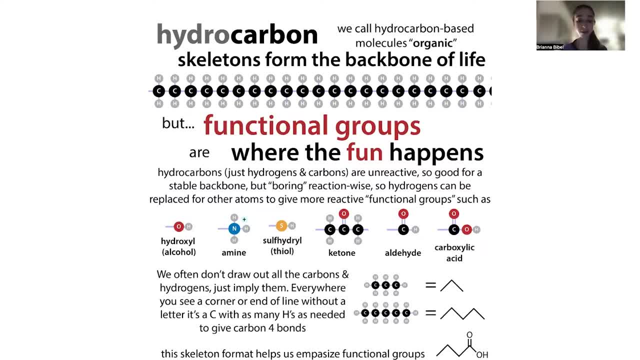 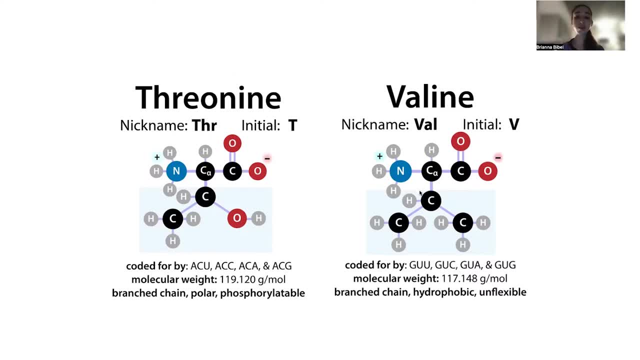 carbon, with hydrogen as a kind of space filler And in the case of valine, as well as the other nonpolar amino acids, we're dealing with hydrocarbons, basically like pure or mostly hydrocarbons. So carbons and hydrogens. 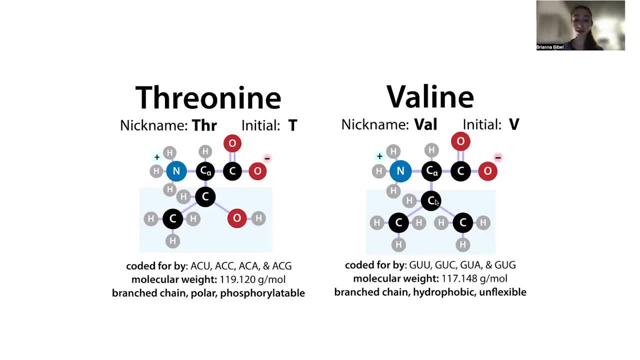 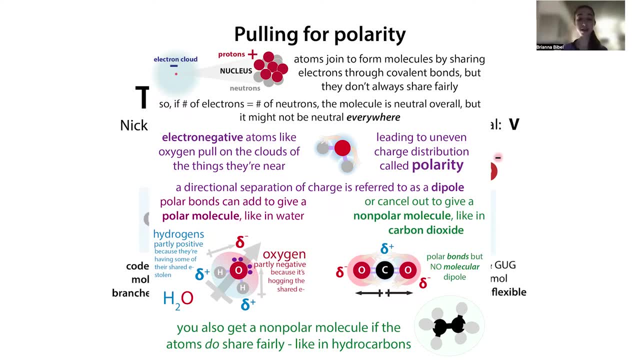 This is going to be kind of blah for reasons what we'll look at: Carbon and hydrogen. they share electrons fairly. more on this in a minute. But basically this is going to be fully like uncharged and kind of just blah And it's going to make it so that it's nonpolar. 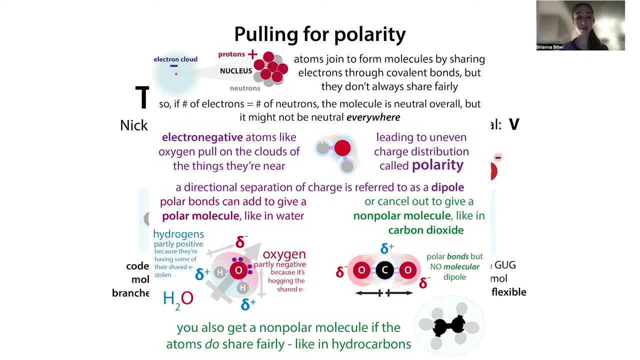 The water doesn't want to hang out with it, Whereas in the case of threonine, we have an oxygen And the oxygen is going to allow it to have a separation of charge. So this is going to be a partially charged, Even though this is neutral overall, you're going to 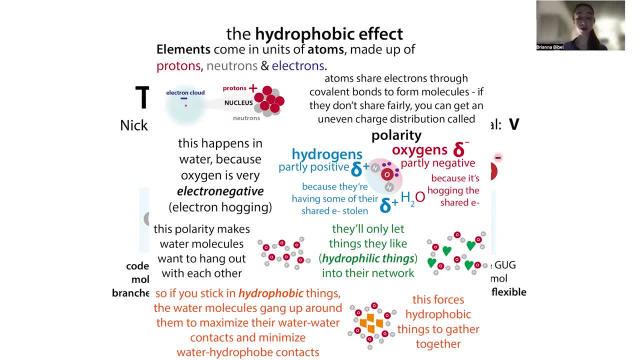 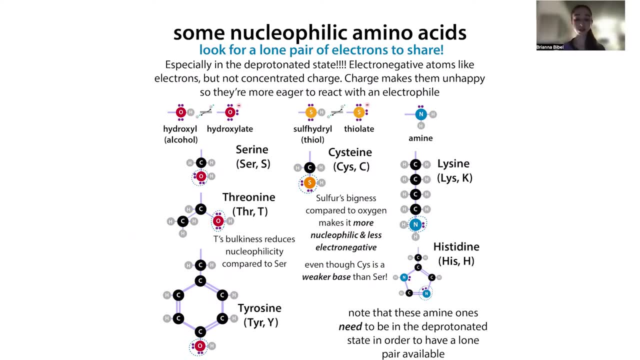 get a partial separation of charge. You're going to have some partial charge that's going to make it attractive to water And this oxygen is also going to make it reactive, because this oxygen is going to be nucleophilic. So, in order to understand what all these terms mean, 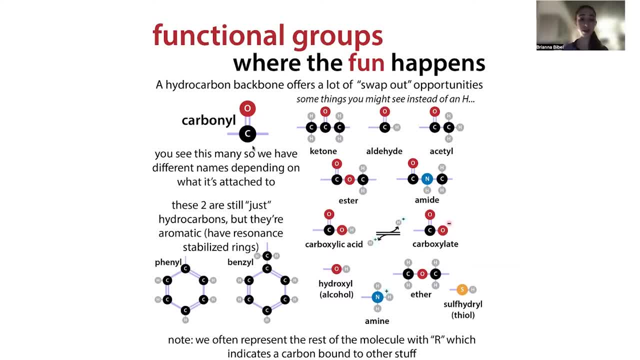 we need to look in a little more detail, beyond just looking at them as these circles, like these letters on them. What are we actually dealing with when we see a C or when we see an O? What we're dealing with are atoms, So atoms are the building blocks of these. 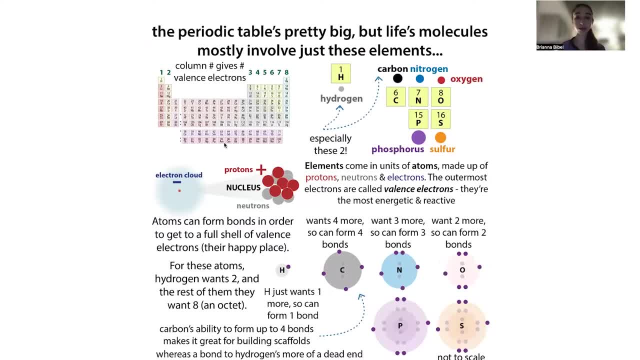 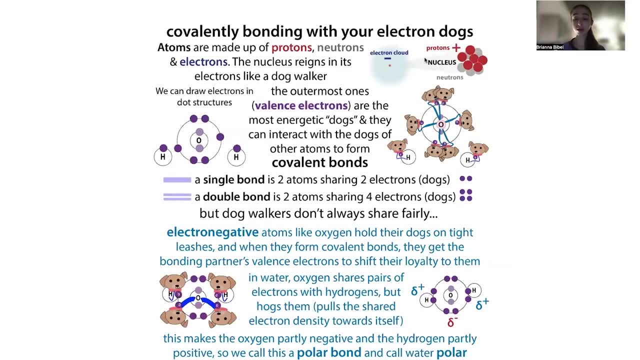 elements and they're made up of smaller parts, these subatomic particles. These include negatively charged electrons, positively charged protons and neutral neutrons. We deal most with the electrons because this is going to be how the atoms are interacting with one another, but the protons are. 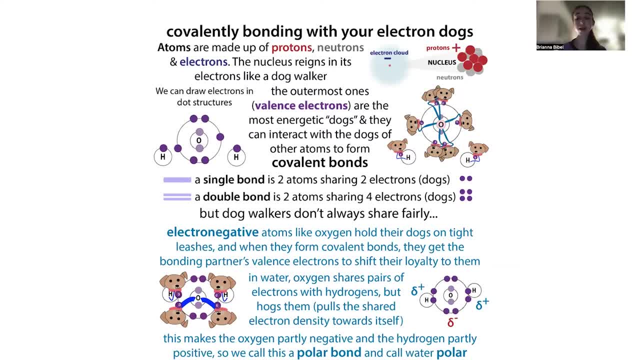 what keep the electrons where they are. So the protons are positively charged and they're glued together by the neutral neutrons hanging out in this dense central core. So you can think of, if you have an atom, the very core of it is going to be the nucleus and that nucleus is going to 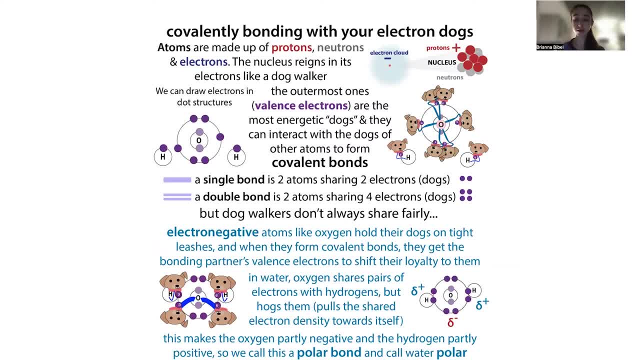 contain the protons, and the protons are going to be positively charged. So at the core of an atom is a positively charged region. Now around that are going to be electrons. Electrons are really tiny and they whiz around and they're. 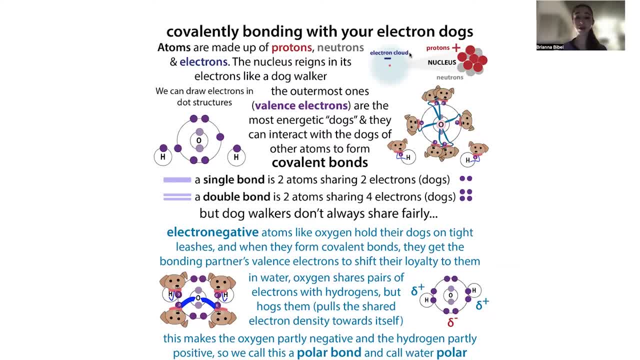 negatively charged. You can never know exactly where they're going to be. We can kind of represent or predict where they're most likely to be and represent these as like orbitals, but we don't know. We can never know exactly, because they're always whizzing around but they don't stray too. 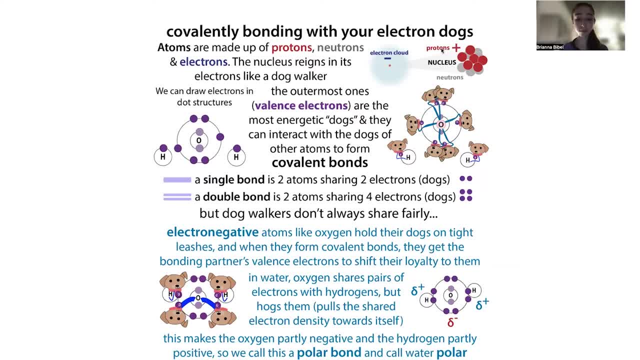 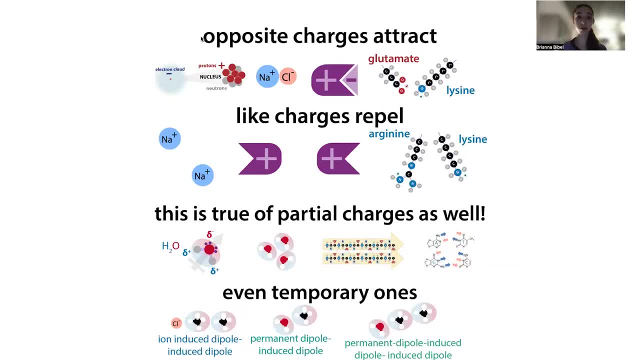 far, because the protons that have the positive pull- you have positive and opposite charges- attract And so the protons are going. the electrons are going to be held around those protons but they're still free to wander about a bit And they can wander about and kind of overlap and get shared with other atoms. 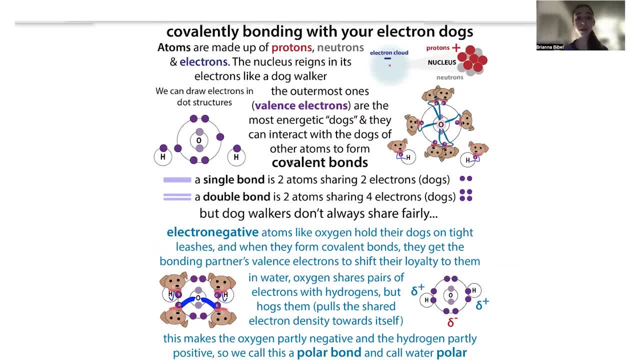 So if you think about, if you think about an atom as kind of as dense central core with this cloud around it. Now, when atoms get close together, what can happen is that if the properties are right of those different atoms, they can kind of merge up part of their clouds When they merge up. 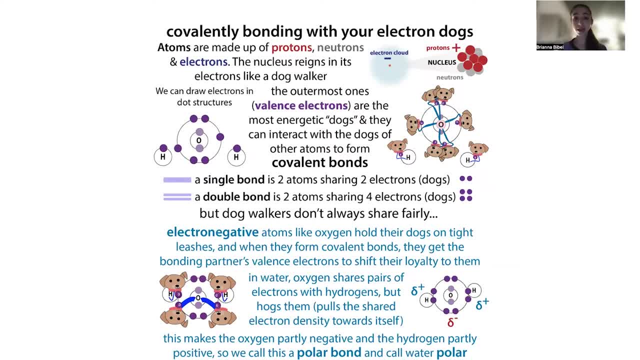 part of these clouds. they share pairs of electrons. If they share a single pair of electron, that forms a single bond, And if they share two pairs of electrons, that forms a double bond. So these are what we call covalent bonds, where you're actually sharing electrons. 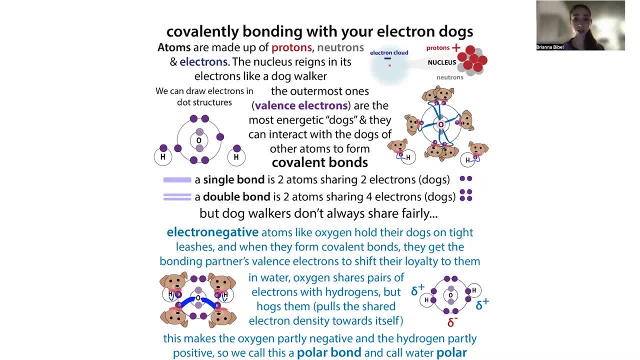 Now they might not always share fairly, however. So this is where I like to get into my analogy of a kind of dog walker. So if you think of a proton as a dog walker and the electrons as dogs, Now the protons are kind of pulling on those dogs with the leash, So that would be like the positive. 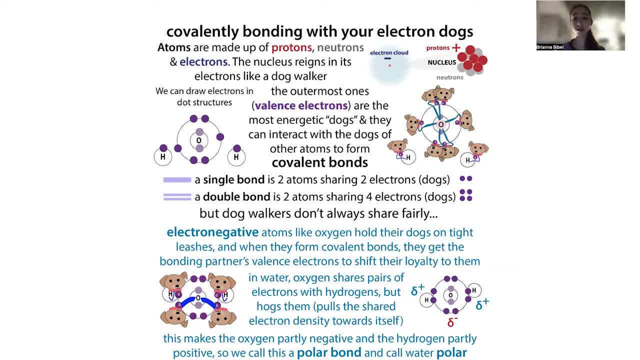 negative attraction. But the dogs have a lot of energy and they might be kind of trying to pull away. So they're kind of pulling on those dogs with the leash. So that would be like the positive. Now some of those leashes might be tighter than others And some of the dogs might be closer held. 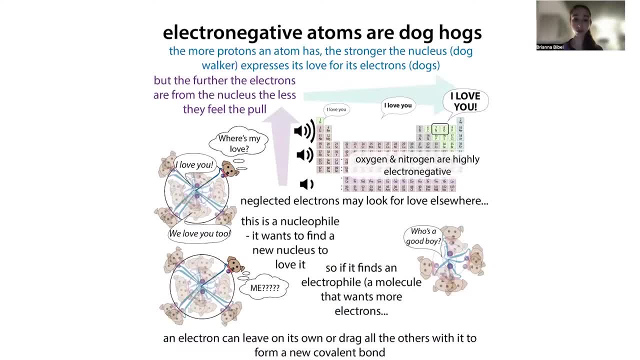 than others. So the closer those dogs are to the proton, the tighter they're going to be held. So the inner electrons in the inner circle are going to be held tighter, whereas the electrons on the outside, what we call the valence electrons- these are going to be more free to wander and to interact. 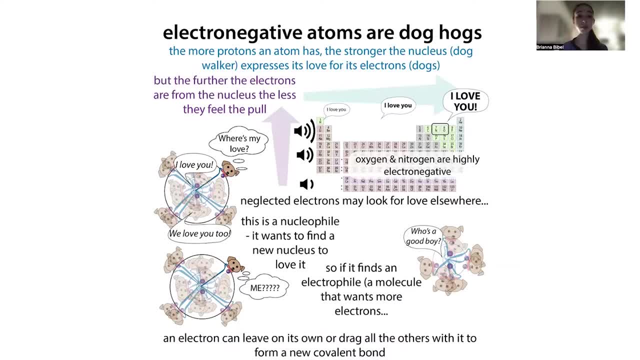 with other atoms. Now, different atoms are going to have different amounts of pulling power, So an oxygen is going to have a tighter leash than, say, a hydrogen or then a carbon. If it has a tighter leash, this means it's going to hold on tighter to those electrons And it's even going to be better at wooing electrons. 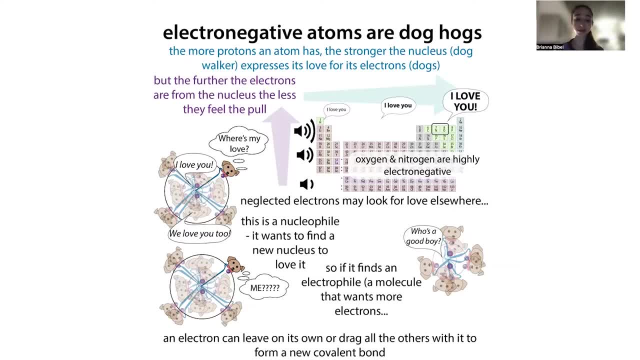 from other atoms. We call these atoms electronegative, And so a key example is oxygen, as well as like nitrogen. So these are going to be electronegative. They're going to pull on the electrons, the electrons that they have. 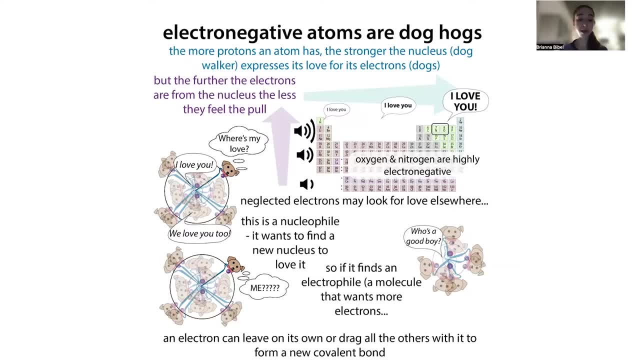 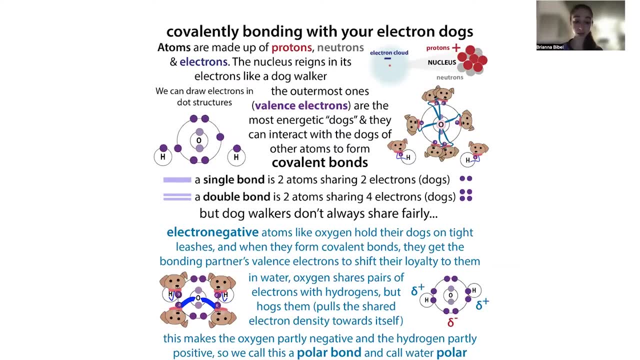 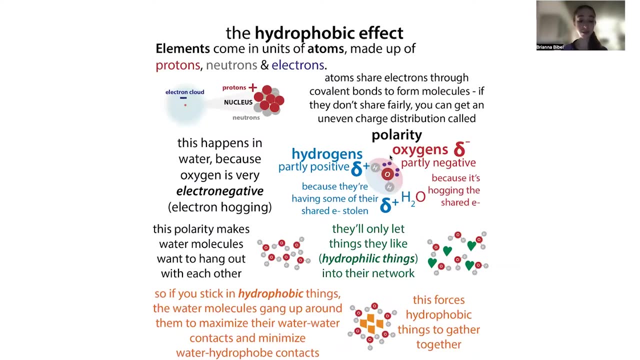 like that they own as well as the electrons that they're sharing with other molecules through those covalent bonds. So if you have a bond where you're sharing electrons between two atoms, such as in the case of these OH bonds in threonine or in the water, what's going to happen is the oxygen being electronegative. 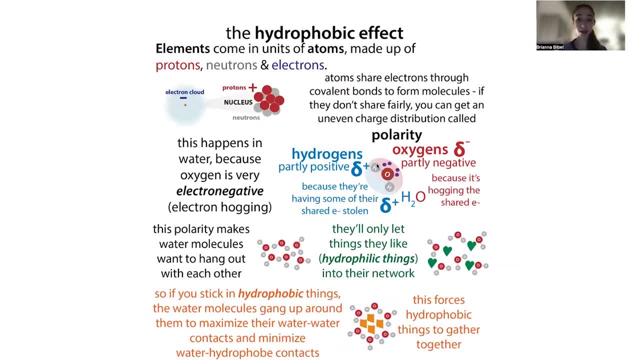 is going to pull the shared electron density away from the hydrogen. The hydrogen, it only has a single proton and it doesn't have a very tight pull, Whereas the oxygen, it's going to have a tighter pull And so it's going to be pulling the electron density away. 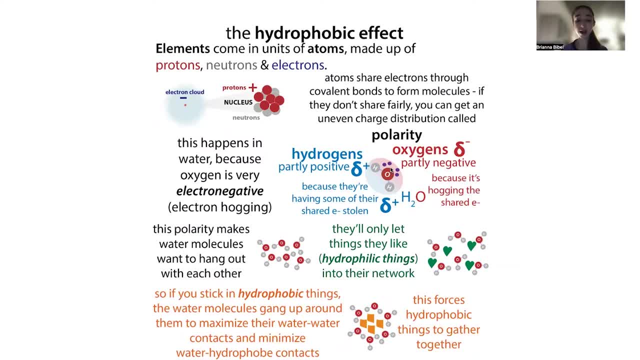 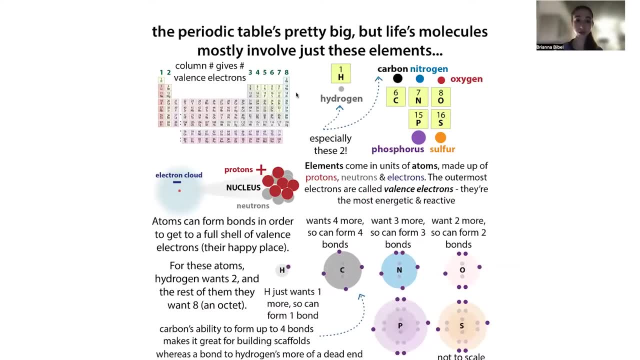 Now, overall, you're still going to have a neutral molecule because you have an even number of protons and electrons. So I forgot to mention this before, but the number of protons is actually going to define the element, and these protons are going to be stuck at the center of the element. 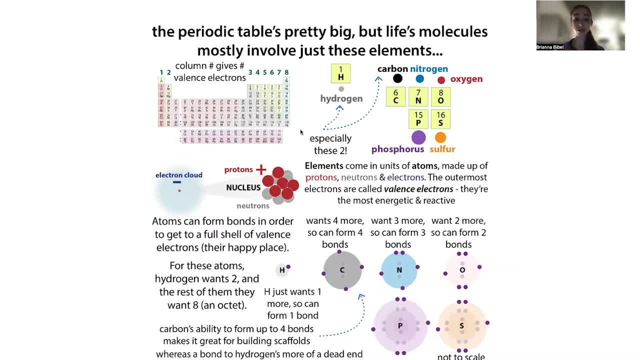 whereas the electrons can kind of shift around. And so if they shift around, so if they're just like right around the right around the the protons, then you have no separation of charge. But if they shift away from those protons, well now the approach where the protons are. 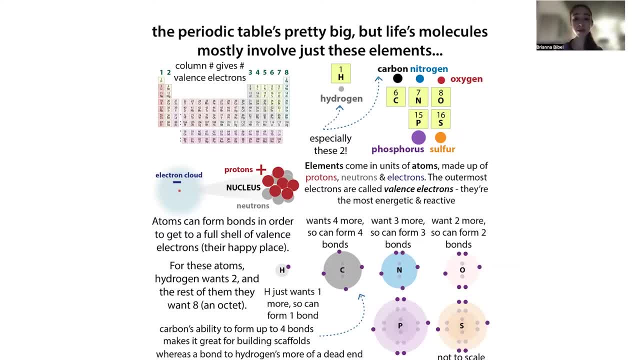 it's going to be partly positive and where the electrons are, it's going to be partly negative. And so if the electrons are hanging out more in a specific area, that specific area is going to be partly negative and the area that the electrons left is going to. 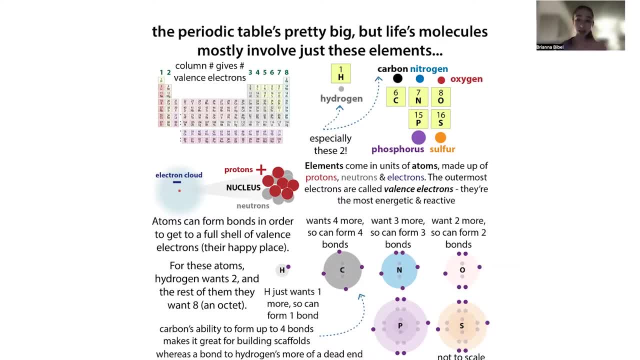 be partly positive. And so if we imagine these clouds as kind of being these shifting shapes, where they're going to be, the electrons are concentrated more in one area or another. well then, that is what we're thinking about when we're talking about polarities, where we have this. 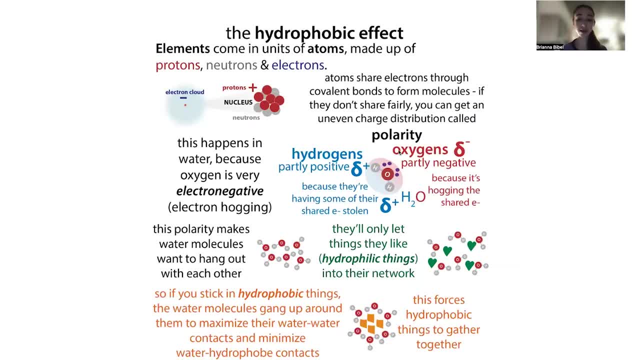 partial separation of charge, where the cloud is going to be heavier in certain parts of the molecule. Basically, you're more likely to find the electrons hanging out there. You're more likely to find electrons hanging out around the oxygen than around the hydrogen, because oxygen is better. 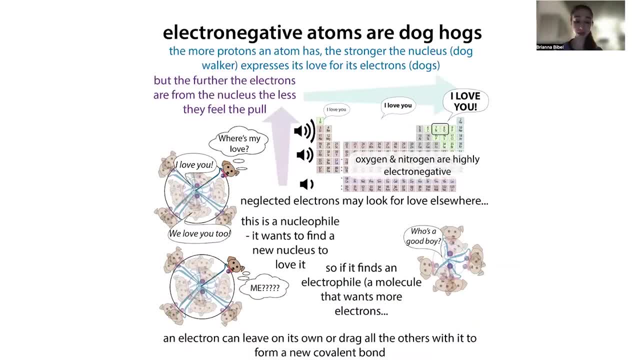 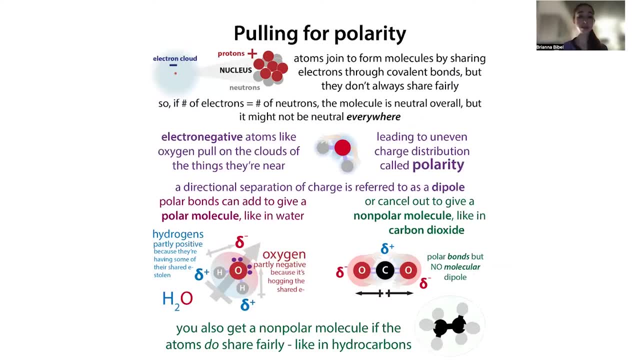 at wooing those dogs. It has a tighter pull over those electrons, the electrons that it owns as well as the electrons that it's kind of like sharing, And so this is where we get this idea of polarity. Now, a couple things about polarity. One is that we can talk about a molecular dipole. 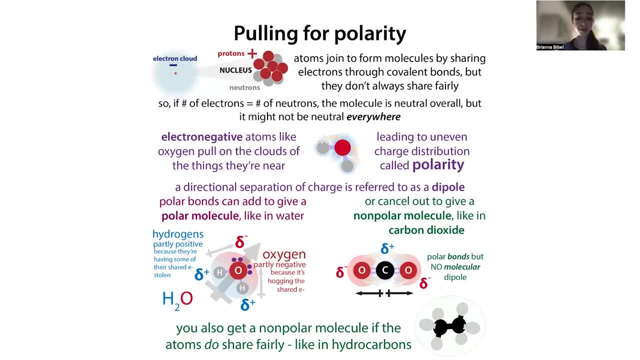 and a dong dipole, So a bond dipole if we have like a polar bond, that's just when we're talking about those electrons that are shared in that one bond, And so you can have a polar bond where you get the separation of charge and that may or may not lead to a polar molecule. 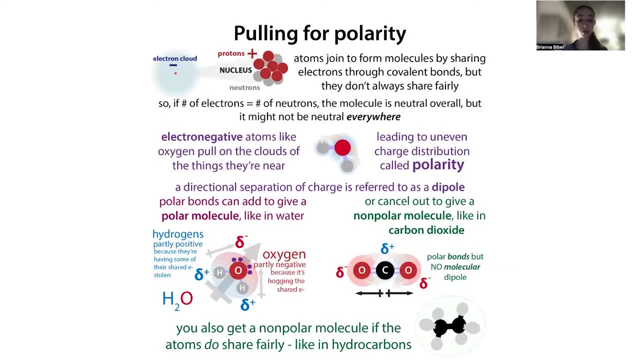 So that may or may not lead to a molecular dipole. So dipole is when we're talking about. you have these two charges that are separated, So this would be like a dipole. That's where we're talking about the leverage agent, the bond dipole. 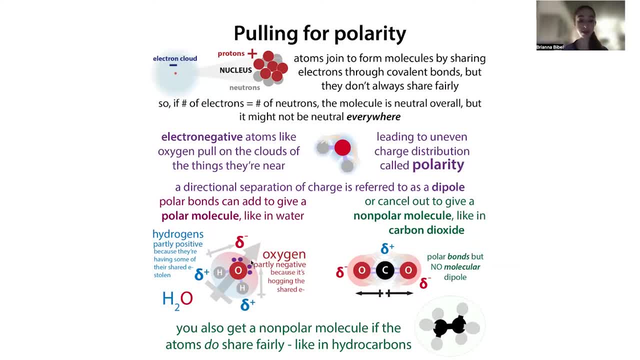 So again, if we have a polar bond and the molecular dipole, in this case you have the molecular dipole because basically you have a separation of charge in the molecule as a whole, not just in that single bond. And this happens in water because you have the oxygen kind of. 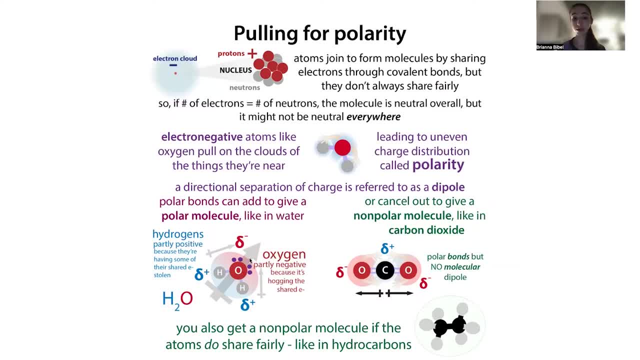 on one side and the hydrogen is on the other side, The oxygen is going to be pulling in both of these directions And so the bond dipoles are going to add together to give you a molecular dipole. Now if you have your dipoles acting in opposite directions- such as the case of CO2, although these bonds have dipoles, although these bonds are polar, the molecule overall is nonpolar because they cancel out. 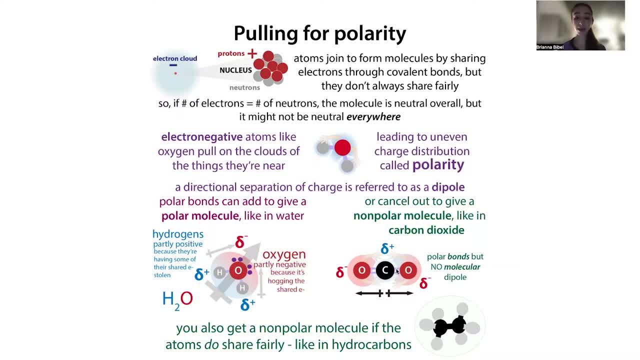 These dipoles cancel out, and so this will have no molecular dipole. So when we're dealing with biochemistry we're often talking about we'll have one part of the molecule be polar, whereas the rest of it might have nonpolar quality. 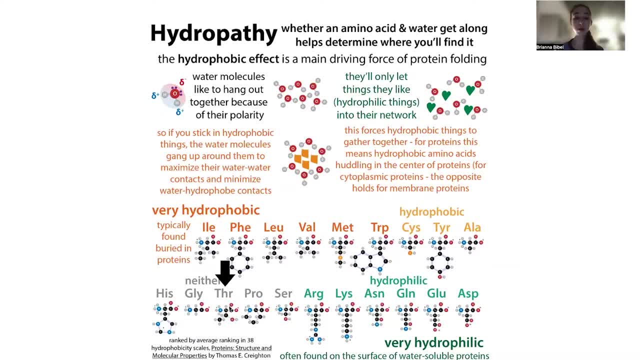 So with threonine, for example, you have this one polar group, but a lot of this is going to be nonpolar, And so the more nonpolar you are, the less water likes you, and the more polar you are, the more water likes you. 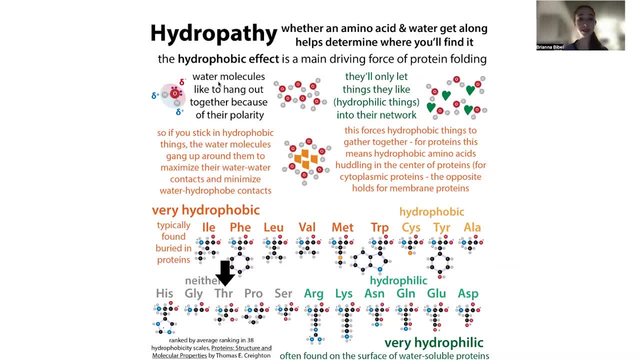 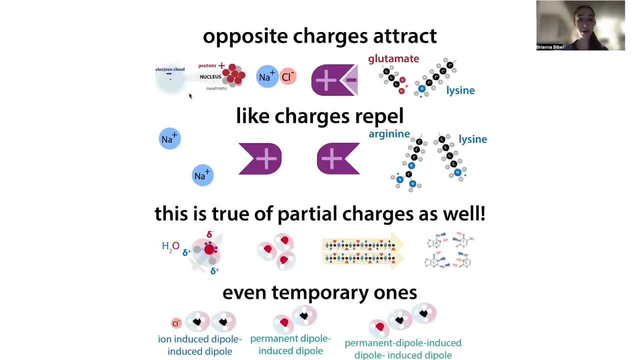 And this is because water is really polar. So we are looking at water as an example of polarity. Because water is such a polar molecule, the oxygen is going to be so poly on those hydrogens and you get that strong dipole. And because we have that core thing in chemistry and biochemistry where we have opposite charges attract even partial charges, then water is going to form these exclusive networks. 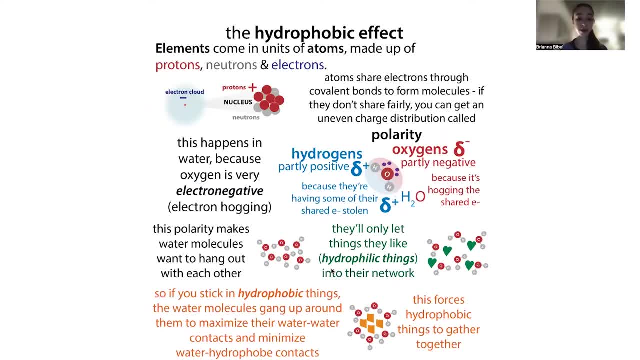 And it's only going to let in other things that are polar or that are hydrogens. So we're going to look at hydrophilic or like charge and stuff, And so basically hydrophilic that means that water will hang out with it and let it into its network. 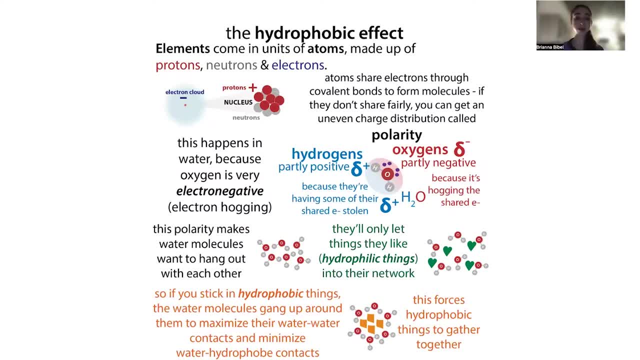 Hydrophobic means that water excludes it and kind of, if water excludes it, those excluded things are kind of going to bunch up together and get hidden on the inside of a protein. In the case of a protein folding, this is, and this is a driving force of protein folding. 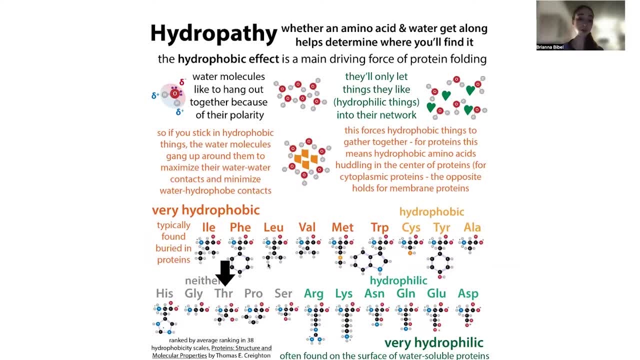 And so if we look at threonine compared to, like baleen, Well threonine is going to be going to be much more hydrophilic than than baleen. So it's still classified as kind of like, neither hydrophobic or hydrophilic according to this one scale, because it still has all that non-polar character because of those CH3 groups. 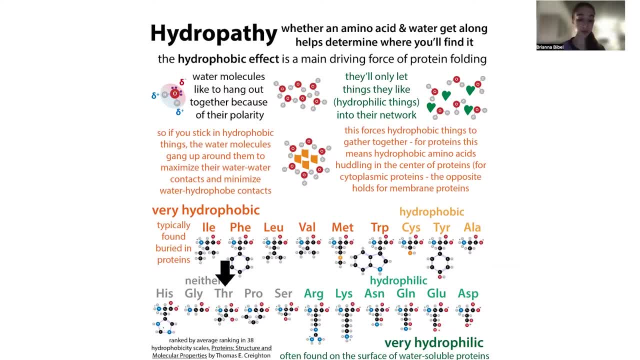 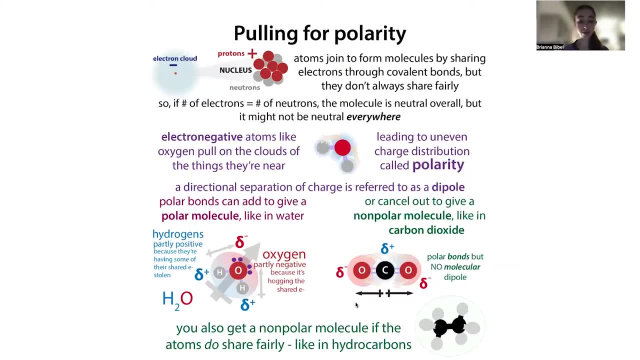 So these CH3 groups, this is just a pure hydrocarbon, And so hydrogen and carbon they share pretty fairly, And so you're not going to Get a polar, you're not going to get polarity if you just have hydrocarbon groups. 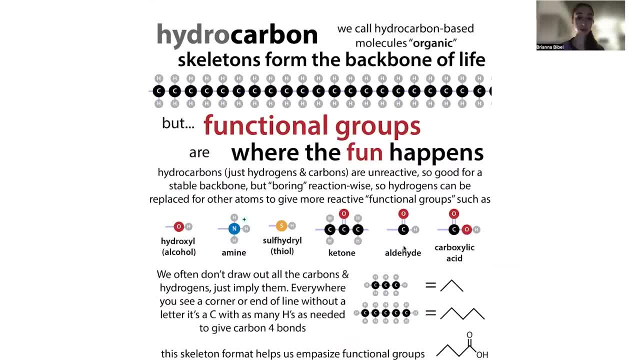 Instead, you need to have some sort of functional group, some sort of swapping out of one of those hydrogen and space fillers for another group with an atom such as an oxygen or a nitrogen or a sulfur That's going to have different properties. 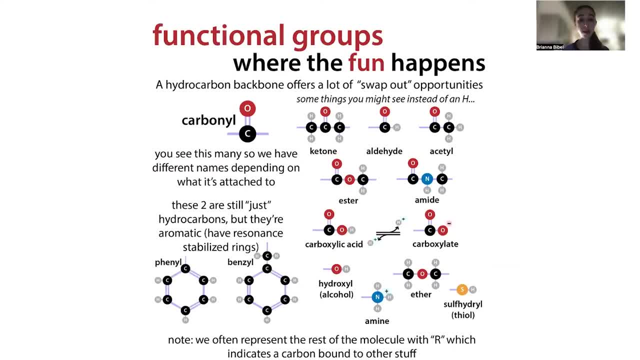 That's going to be have more pulling power. And so this is what we see with the case of Threonine, where we have this hydroxyl, this alfohol or OH group, where we saw how oxygen was going to be really electronegative. 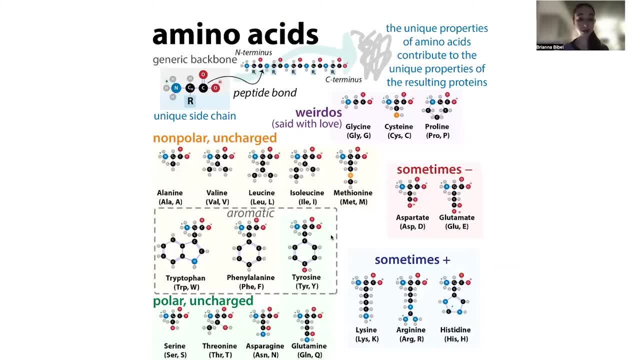 Now. so if we look at our amino acids charts, we can see that threonine is not the only one with an OH. You also have serine and tyrosine that have these hydroxyl groups, And we'll get more into this, but this is going to allow all three of these to be phosphorylated. 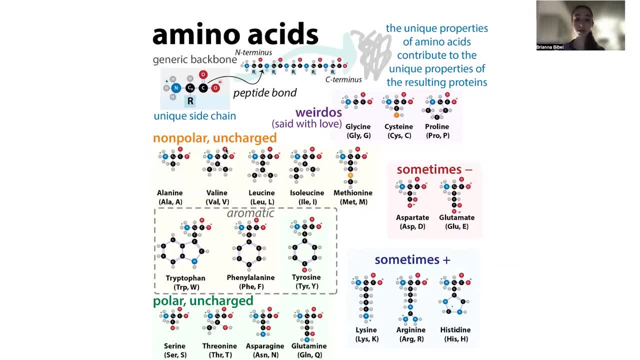 If we look at our non-polar amino acids, Well, here we're seeing basically strictly hydrocarbons for the most part, So just carbon and hydrogen, which, remember, they're sharing those electrons pretty fairly because they have similar electronegativity. 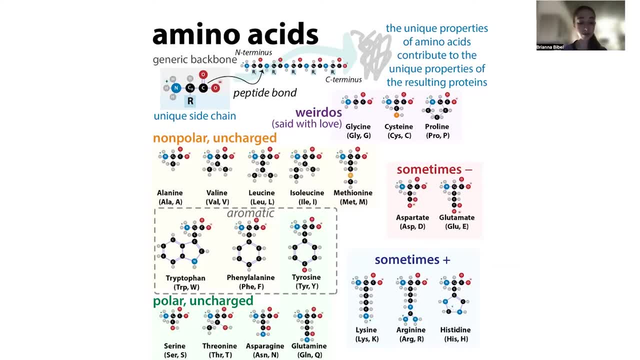 So they have a similar pull over the electrons, And so you don't get that separation of charge, You don't get that polarity when you don't have. when you just have this like pure neutral molecule, no partial charge or anything, Well, that's going to be really boring for the water. 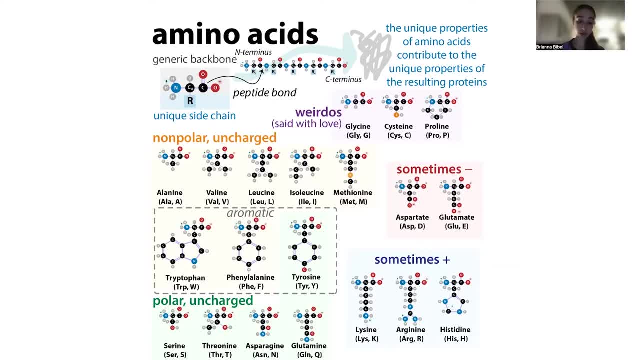 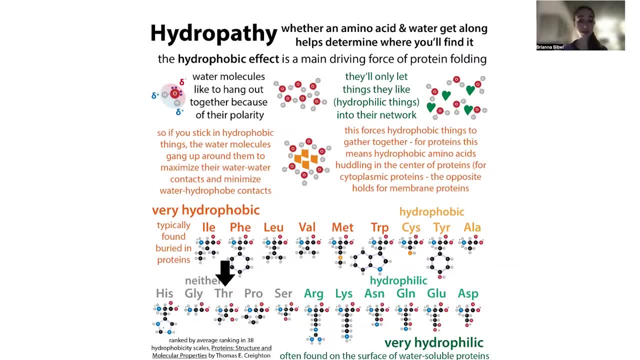 So these are also going to be hydrophobic, Whereas when we talk about these polar molecules, the more polar they are, the more hydrophilic that they are. but it's the spectrum, So we can't just say, oh, if you're, if you're polar, that means you're going to be really hydrophilic. 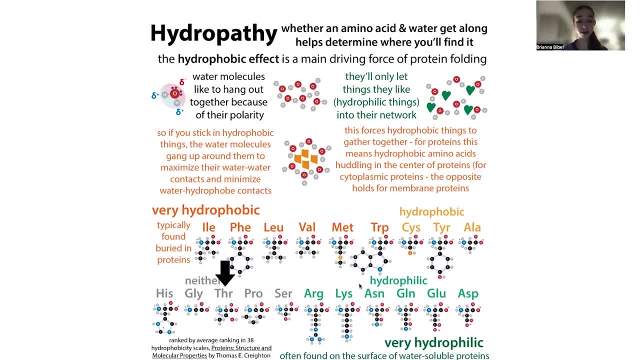 Instead, it depends on, like, how polar they are as well as so, like, how much of it is hydrocarbon versus how much of it is actually having a partial charge, And if you have A full charge, well, that's even better, And so we'll get more into this later, when we talk about the amino acids that are charged. 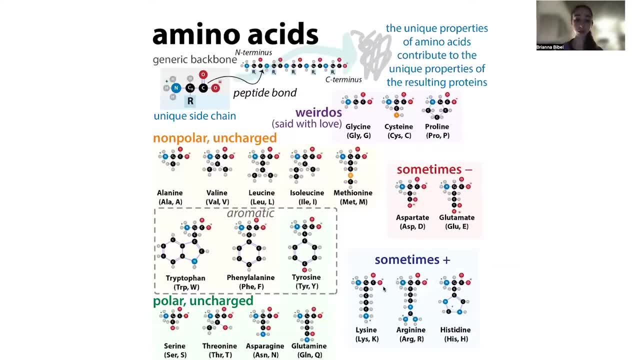 And so sometimes you'll see amino acids classified as like polar, non-polar, uncharged, or polar uncharged as well as charged, And so we'll get more into the charge once later. but when we're dealing with threonine, we're dealing with a polar and uncharged because it has no full charge. 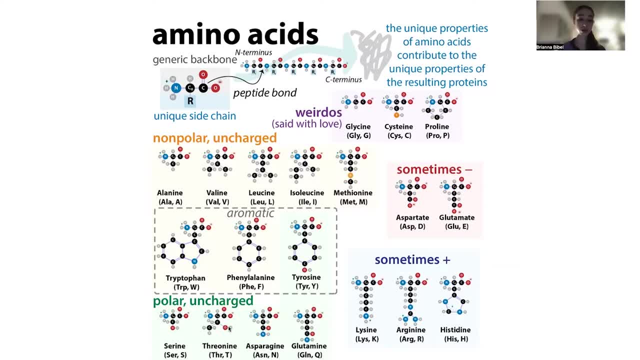 It just has that partial charge, and it has that partial charge because of that OH. You'll see that asparagine and glutamine- these are also polar uncharged, but instead of an OH they actually are going to have an amide group. 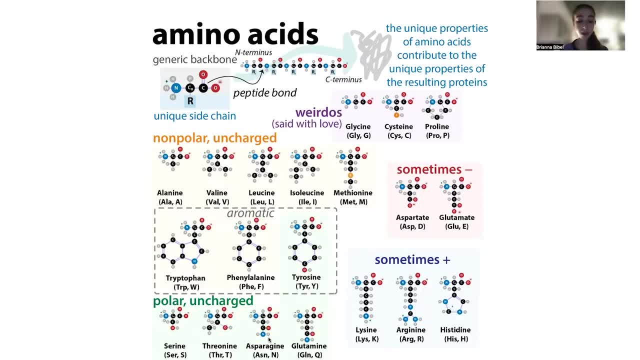 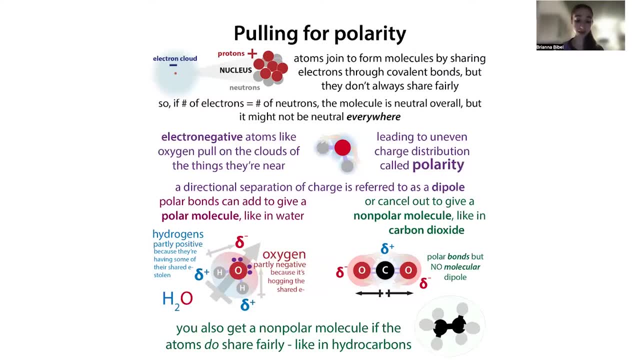 And so they're going to have an oxygen, a nitrogen, and we'll get more into them later. But all of these are going to be examples of polar molecules And because they have that polarity, they're going to be able to hang out with water. 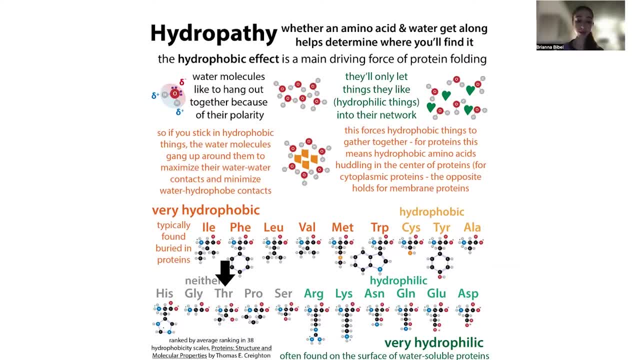 And so you're more likely to find them on the surface, And so you're more likely to find them on the surface of a protein. but in the case of like threonine, you still have a lot of hydrophobic character because of those hydrocarbons and stuff. 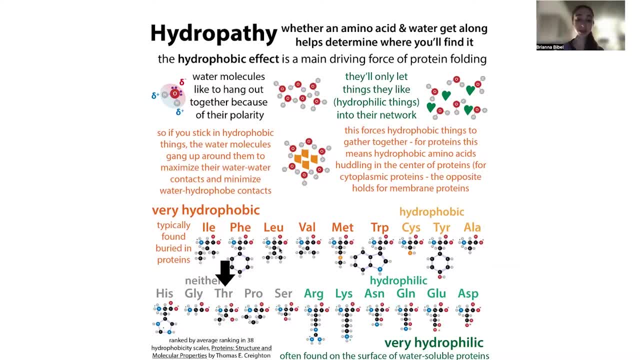 And so it's not going to be that hydrophilic, but it's not going to be nearly as hydrophobic as lucilin and valine, So you can kind of find it more places. In addition to making this amino acid more hydrophilic, the oxygen is also going to allow it to do other things and allow for post-translational modifications. 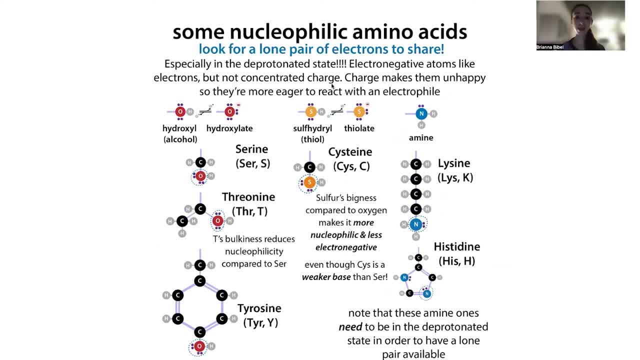 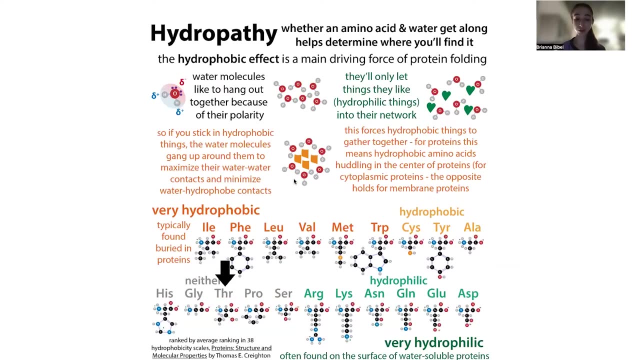 Because oxygen not only is electrophilic, it's nucleic. Now, because oxygen has that electronegativity, it's going to allow threonine to play nicer with water, It's going to allow it to be polar. So when you think of polarity, typically, what we're dealing with at the core, we're dealing with that separation of charge. 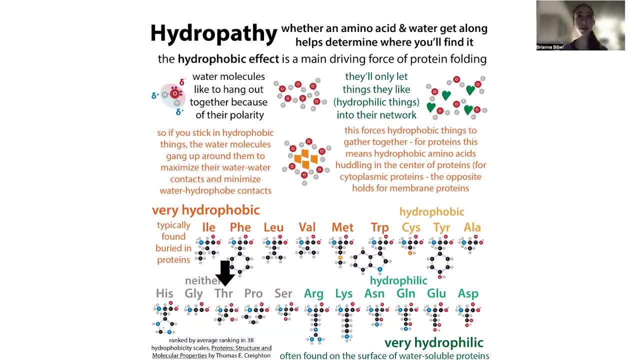 But in practice and in Like, as a consequence that's going to affect the hydrophilicity, hydrophobicity. So the more polar something is, the more likely it is to hang out with water, the more likely you are to find it on the surface of a protein. 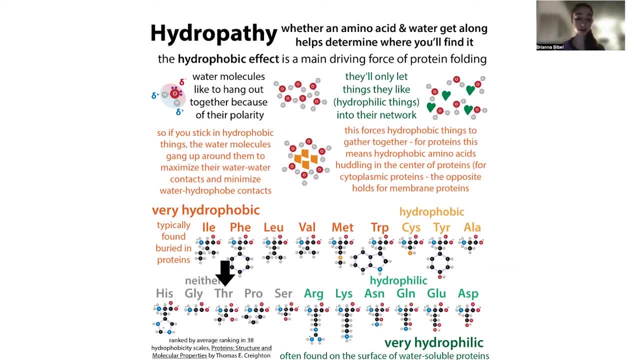 But not all polar molecules are created equal and not all electronegative atoms are created equal, And what happens in this case of a hydroxyl group is it's also going to be very nucleophilic, And so nucleophilicity- this is another term we need to talk about. 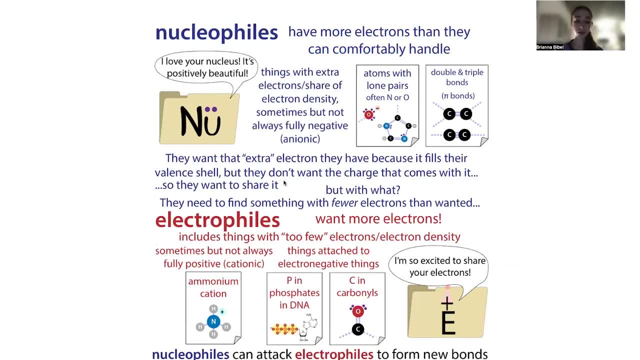 Basically, a nucleophile is something that has more electrons or electron density than it can handle And it's looking for something positive to share with. And so, if you think about the case of the dog walkers, it's like the dog walker, It really likes dogs, so it keeps finding dogs or keeps signing on to walk dogs. 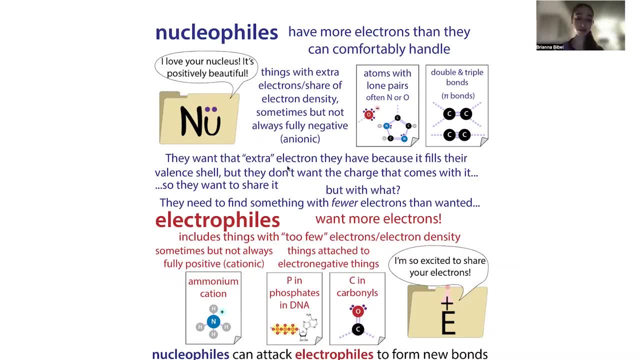 But then it has more dogs than it can really handle, but it still really wants to hang out with those dogs. So it wants to find another dog walker to help, And this is going to lead it to seek out electrophiles which are going to be like dog walkers, looking for dogs. 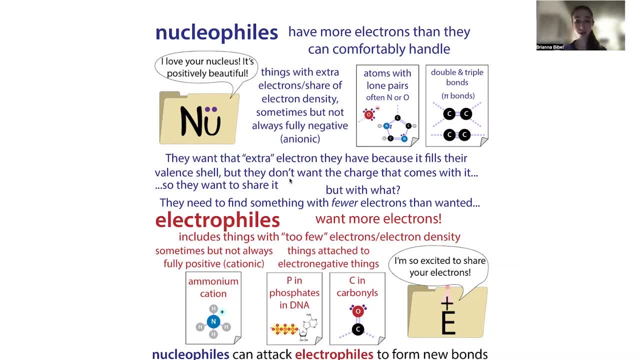 These are going to be atoms that want more electrons, So they have too few electrons or electron density, And so when a nucleophile attacks an electrophile, this is a way that you can form new bonds, such as through a substitution reaction. 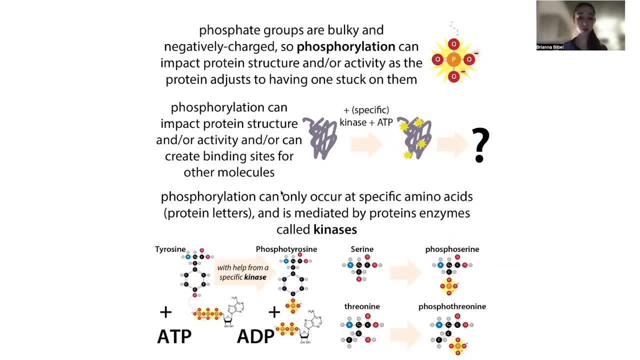 And this is what we're going to see when we look at the case of phosphorylation. We're going to have that hydroxyl group of tyrosine or of serine or of threonine attacking. So this would be a nucleophile attacking an electrophile, in this case a phosphate group in ATP. 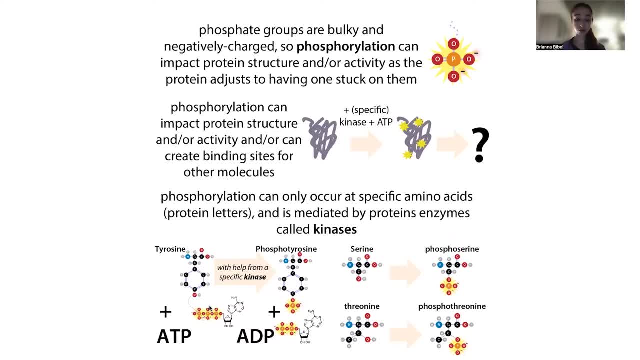 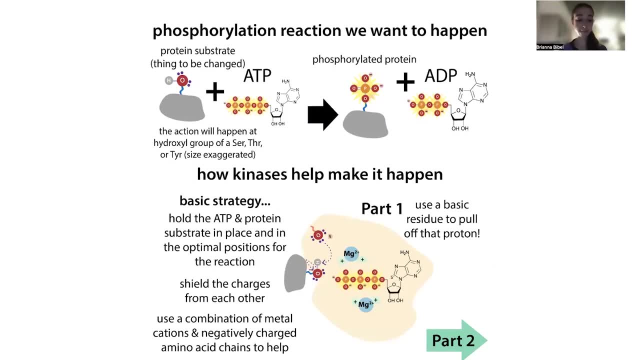 to get this phosphoryl group transferred in a substitution reaction, And we'll look at how enzymes- so reaction helpers called kinases- are going to help make that happen. But first we need to understand the study of electrophiles and nucleophiles a little better. 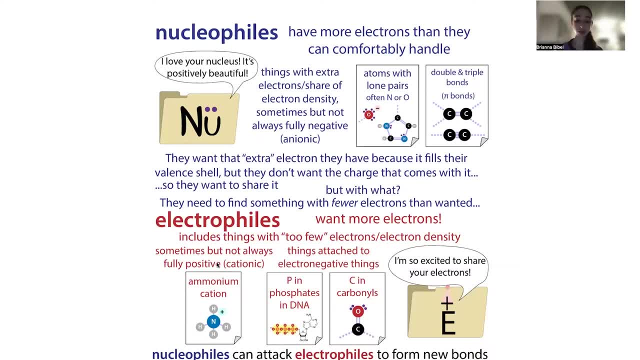 So a nucleophile, remember this- is something that has more electrons or electron density than it wants. You can kind of remember this as thinking of like a little like dotted electrons over you as like a kind of smiley face. This is how I remember a nucleophile. 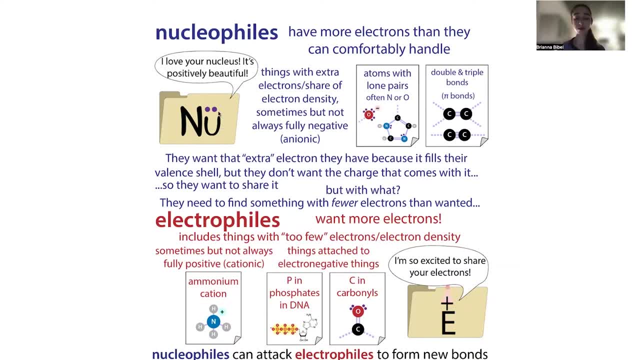 But one way. The other way is that it goes to nucleophiles looking for nucleus, because that's where the positivity is. So nucleophiles are sometimes negatively charged, but not always. They're going to typically Be an electron negative atom because, remember, the electron negative atoms are going to have a tighter pull over those electrons. 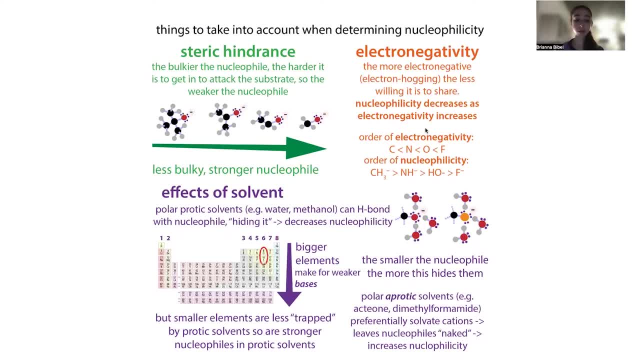 So they're going to have more electrons hanging out near them. But remember, they have that limited number of protons. They have that proton, the number of protons that defines elements. So that's fixed. But the number of electrons can vary and the electrons can. more electrons can hang out with it than the protons can handle. 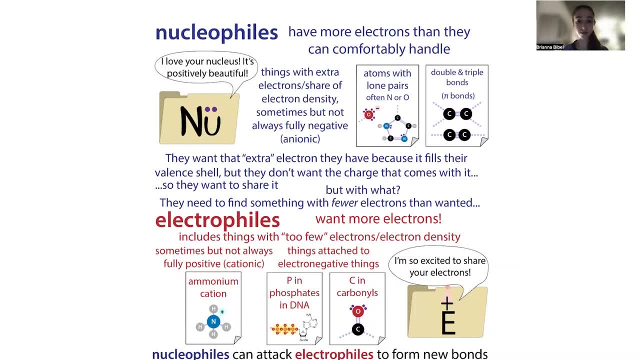 And this leaves you with a situation where you have a strong nucleophile, And if you have a strong nucleophile you can handle it. But if you don't have a nucleophile, it's going to want to seek out an electrophile. so an electrophile is looking for electrons. 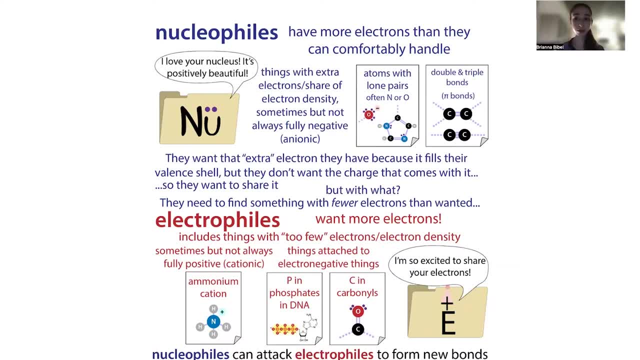 So the nucleophile was looking for a nucleus, because the nucleus is where the protons are. That's where the positivity is. The electrophile is looking for electrons, So they're looking for more of that negativity. So electrophiles are sometimes, but not always, positively charged or they're partially positively charged. 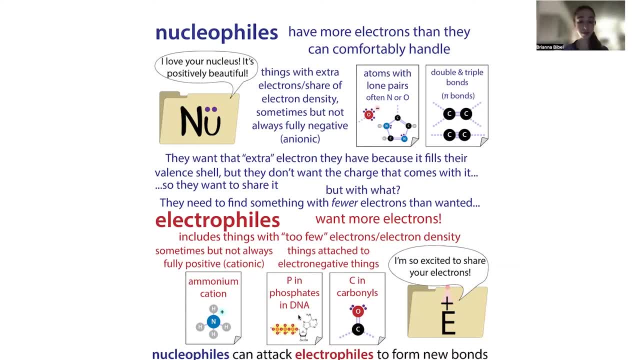 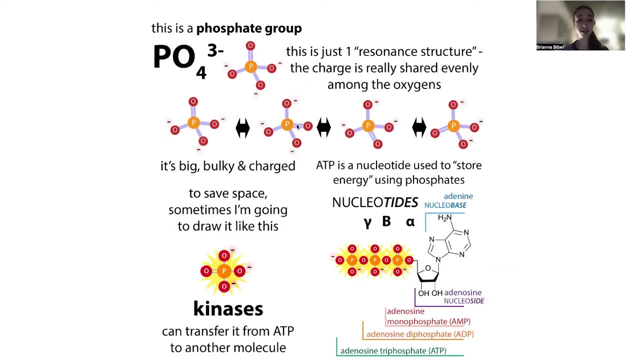 And so a key example of this is going to be the phosphate, The phosphorus in a phosphate. Now, at first glance this might seem kind of confusing because, well, if you look at a phosphate group, it's negatively charged, but this is going to be a negative overall charge. 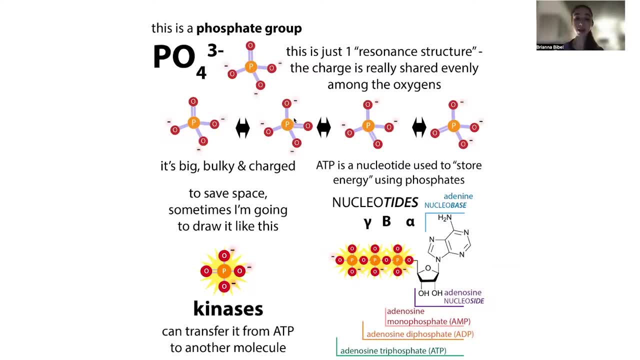 And what happens is that oxygen- remember oxygen is really electronegative- is going to be pulling away the electron density from this phosphorus, And so this is going to leave this phosphorus partly positive, even though these oxygen groups are partly negative. 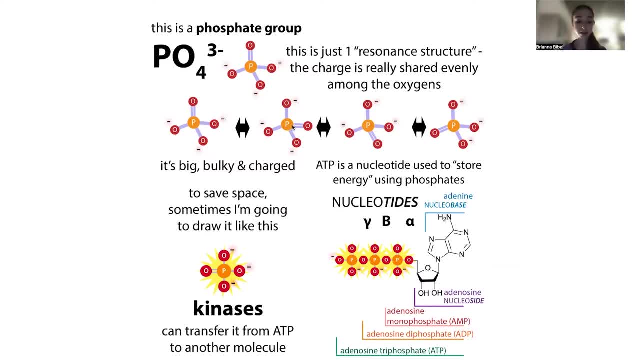 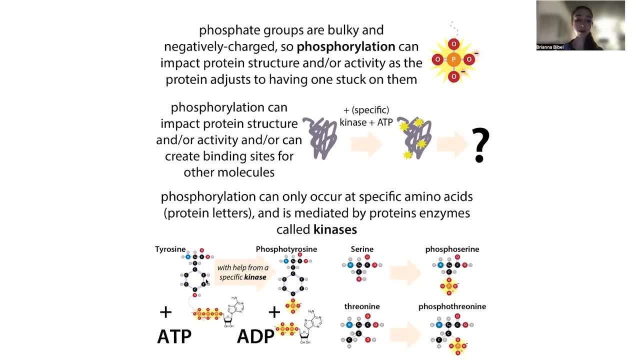 And so this phosphorus is going to be electrophilic and it's going to be vulnerable for attack, And this is what's going to happen. is that the hydroxyl group, this oxygen here, this oxygen is nucleophilic. 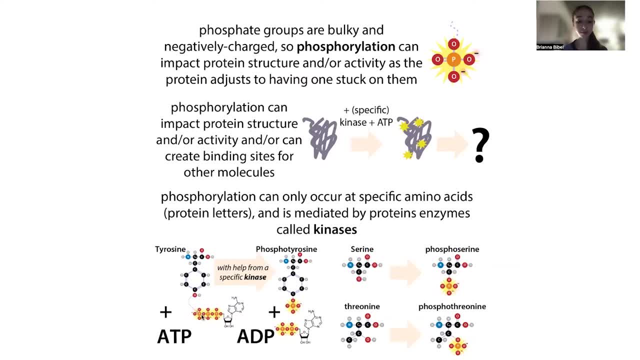 It's going to attack that electrophilic phosphorus, and then that's going to make it so that there's two bonds to the phosphorus, And so the ADP is going to get kicked out, leaving you just with this phosphorylated protein, this phosphorylated amino acid. 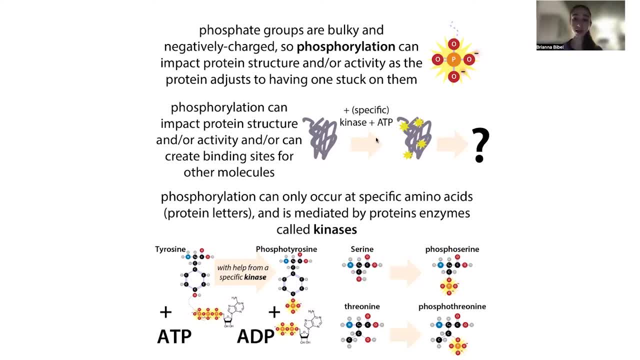 And the consequences of this. well, it depends. Because this group is big and bulky and negatively charged, it can affect, it can kind of make the protein have to shapeshift or undergo a conformational change in order to accommodate things. 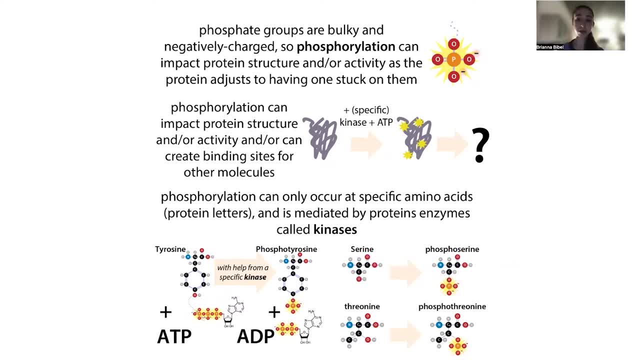 And it can also open up new binding sites and opportunities on the surface of a protein, because you're allowing changes, so it can influence what a protein interacts with and how that protein functions. And so this can be used To activate and inactivate various enzymes or reaction helpers to regulate, regulate cell signaling, regulate metabolism, so the making and breaking of molecules. 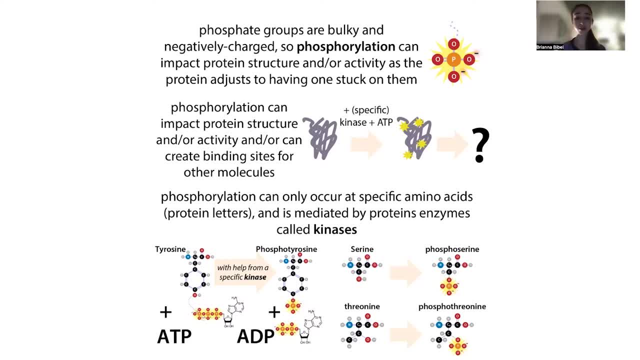 So you see phosphorylation a lot in biochemistry and you can only see it in specific with specific amino acids such as tyrosine, serine and threonine, because they have that. they have this oxygen group, You can also this hydroxyl group. you can also get phosphorylation sometimes with histamine. 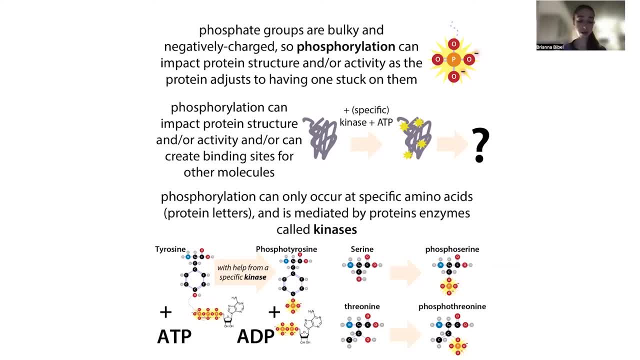 And this happens more in bacteria. It's not exactly known how common it is in like in our cells, in non-mammal cells, in eukaryotic cells, so like non-bacterial stuff, because it's really hard to study. 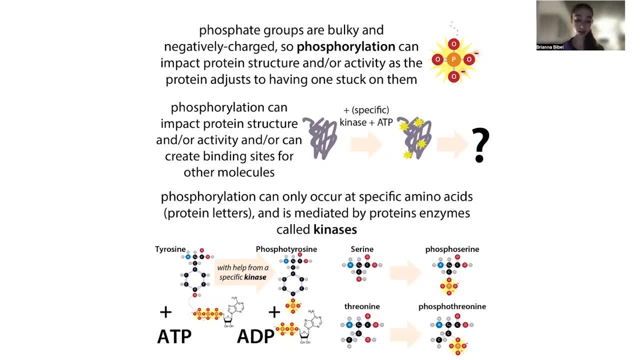 But it's a growing area of research and there it can happen on one of the nitrogens. But in the case of serine, threonine and tyrosine, we're dealing with it happening from the hydroxyl group. 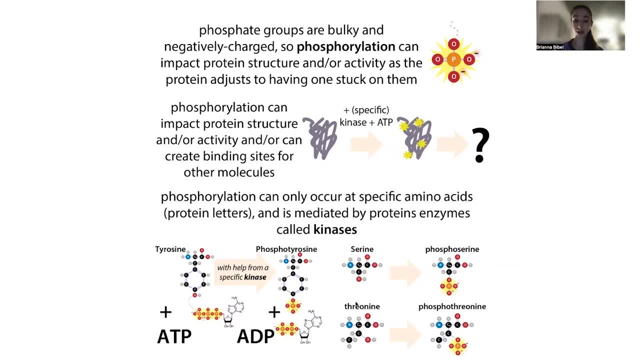 And so, remember, these are the three that have this alcohol, that have this hydroxyl group, And these are the three that have this hydroxyl group. And these are the three main ones that we talk about when getting phosphorylated, And this phosphorylation is going to be aided with the help of a kinase. 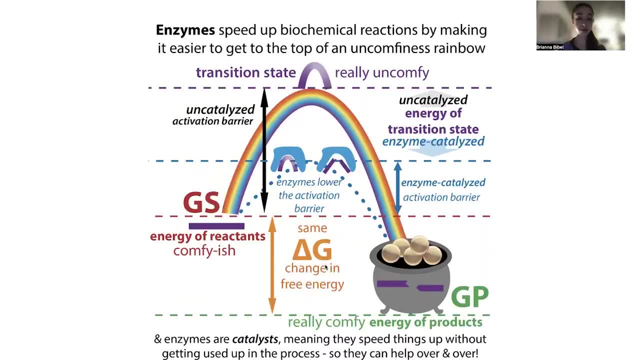 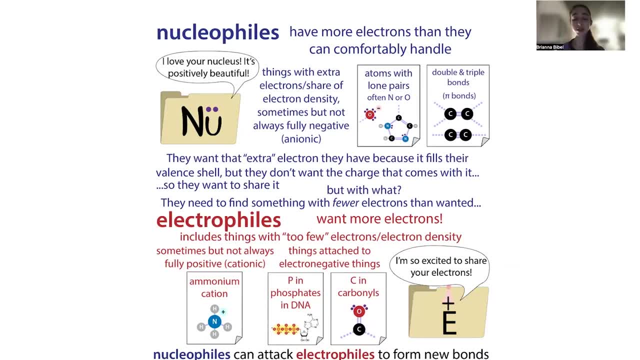 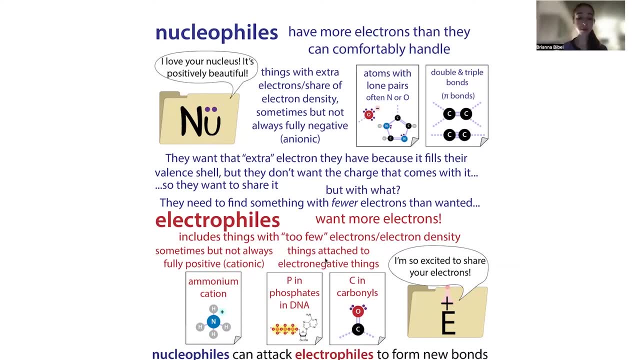 each other, then I'm going to be able to tell the others there. So the enzyme can kind of help facilitate bringing them together, holding them in the right orientation and providing it, making it so that the nucleophile is more nucleophilic, the electrophile is more electrophilic, such as: 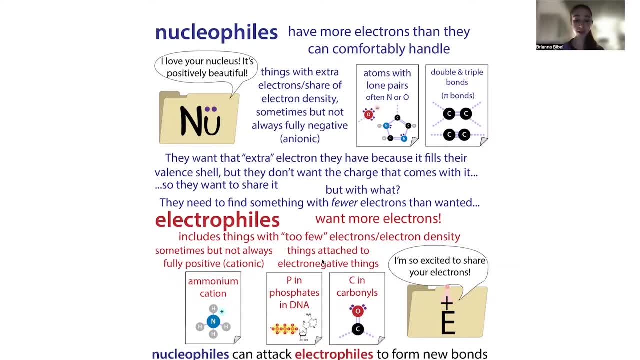 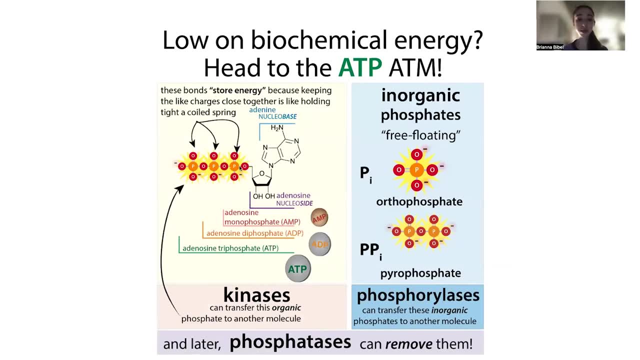 by, say, influencing where those electrons are hanging out more. And so this is what we see in the case of a kinase. The kinase is going to take a phosphoryl group from ATP, so from adenosine triphosphate, and transfer it onto the protein, But the protein is actually going to be the one. 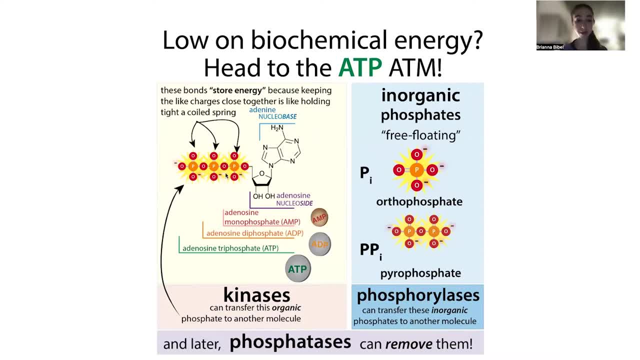 attacking The kinase is just going to help make it happen. A quick naming thing. So basically this is ATP, adenosine triphosphate. This is also an RNA letter, but it serves as an energy currency as well, kind of like an energy arcade token. Your bodies can take a lot of different. 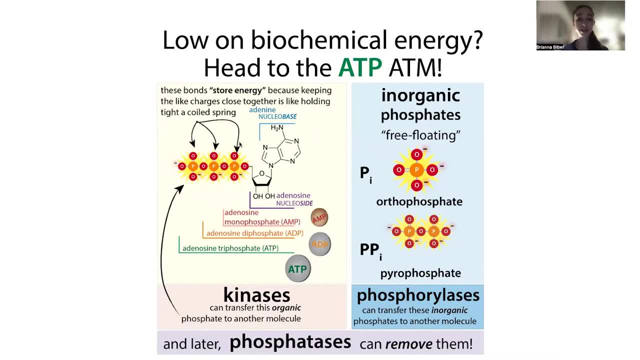 nutrients break them down into, into energy that is stored in the form of ATP that you can then cash in in different reactions. And these phosphates, in addition to being used for energy, these phosphate groups, can be used to modify proteins or other molecules with the help of kinases, And so a kinase is going to. 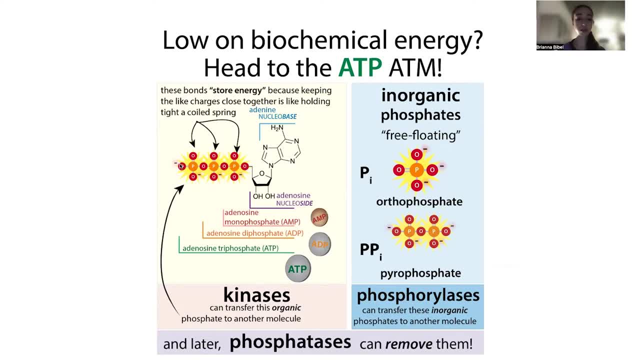 transfer this last phosphate group, this gamma phosphate, onto a protein or onto another molecule. So not all. some kinases work on proteins, some protein kinases, others work on other molecules, But they're going to transfer this gamma phosphate group. Technically this is a phosphoryl group that 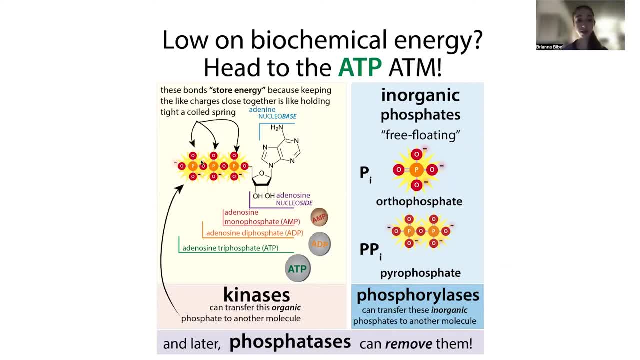 they're transferring because they're not going to be transferring. they're going to be transferring three of the oxygens, but not the fourth one. The fourth one is going to be, as we'll see, coming from the protein in the case of a protein kinase. So the oxygen of the protein is going to. 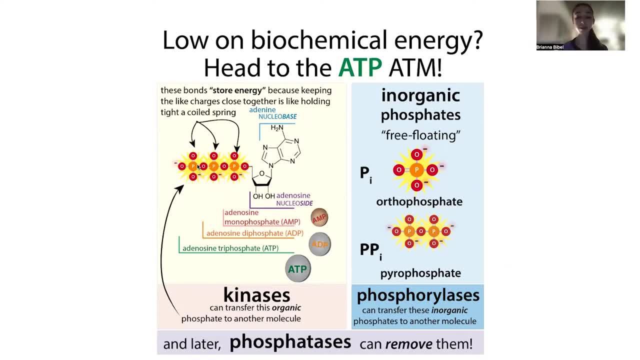 be attacking the phosphoryl group of ATP and the phosphate group, the phosphors of ATP. so you're transferring a phosphoryl group technically, not a phosphate. You're transferring a phosphate group which would be having all four oxygens. But typically we just say: 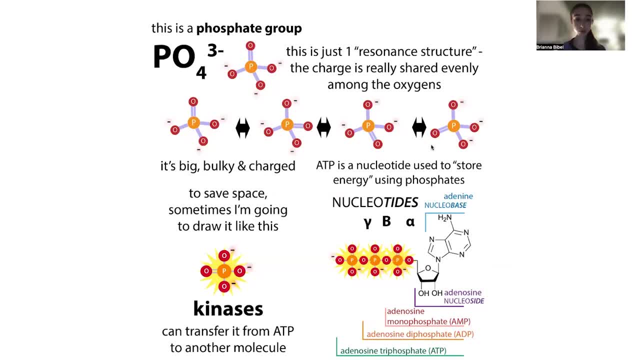 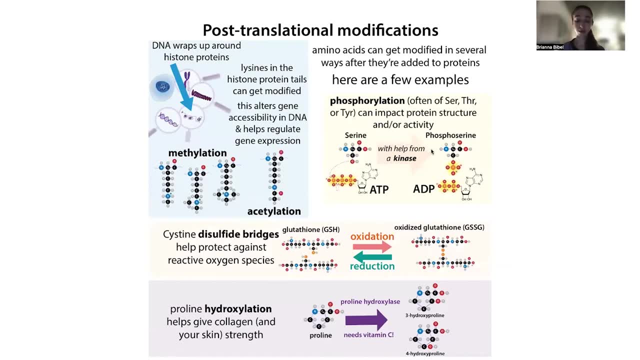 like a phosphate group, But technically it would be a phosphoryl group, And this is one example of post-translational modification. And so remember, this is modification that's happening to a protein after it's been translated. So, after all those individual amino, 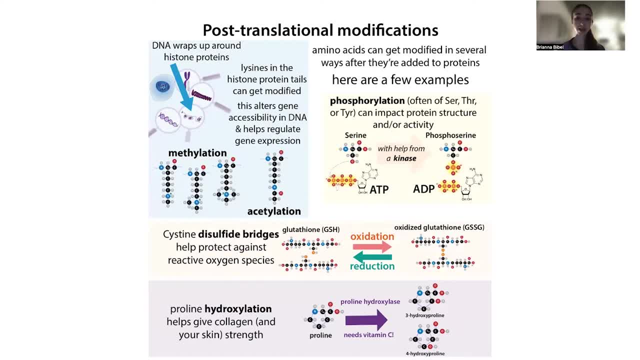 acids are linked together. now this modification is getting added. It's not going to be added before the amino acid is actually added into the protein. So it's not going to be added before the amino acid is actually added into the protein. So, although we have this set of amino acids, like those 24 amino acids that can get genetically, 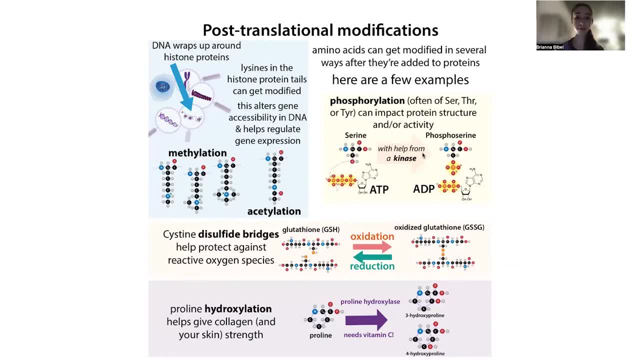 encoded so that the ribosomes can incorporate when they're making a protein. we have more diversity. that can happen thanks to some of these amino acids being able to be modified in ways such as phosphorylation or, as we'll look at later, methylation and acetylation and hydroxylation. 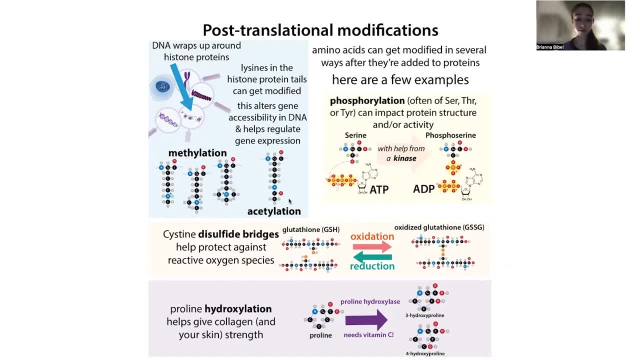 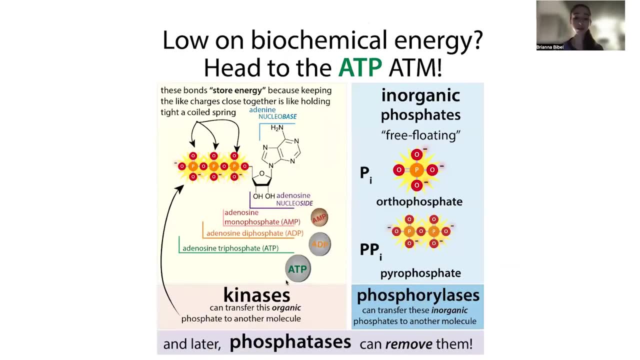 and things like that. But today we're dealing with phosphorylation, and when we talk about methylation here we're dealing with kinases, which are the enzymes that add these phosphate groups, And then there are also phosphatases, which remove the phosphoryl groups. 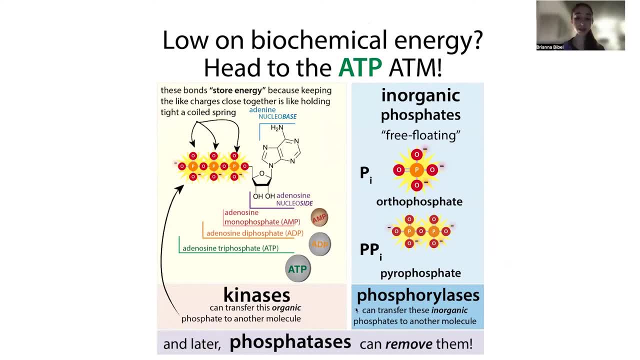 Just another quick note is that phosphorylases- these can transfer inorganic phosphates to another molecule. So basically inorganic phosphates, they're not coming from ATP, they're just kind of free-floating. But most of the time we're dealing with kinases where the transfer is coming. 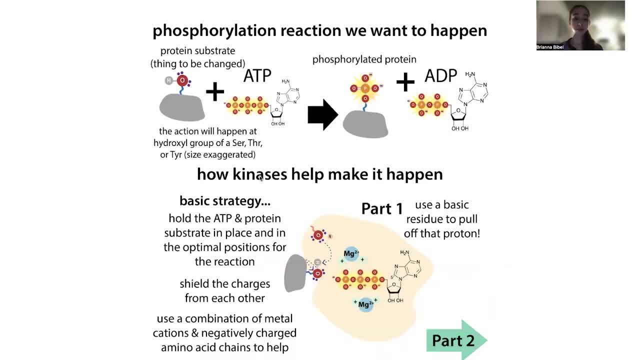 from an ATP molecule. Okay, so let's go back and let's look at the idea of our nucleophile and our electrophile and what's actually happening in phosphorylation. So we have from nucleophile- remember that's something that has more electron density than it wants- and an electrophile is something that. 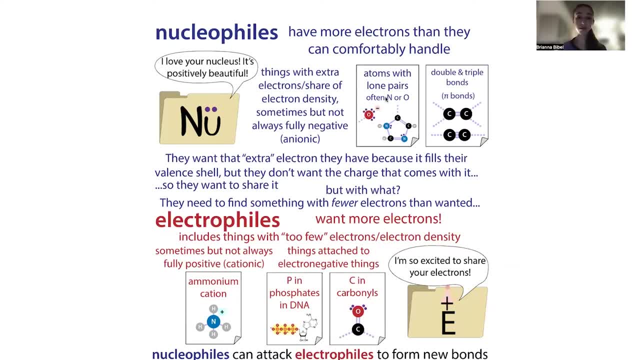 wants that electron density. So when I'm talking about the nucleophile, here we're going to be- in this case we're going to be dealing with the oxygen. Other times you're dealing with nitrogens. What's common a lot of times is they have this lone pair of electrons and this lone pair. 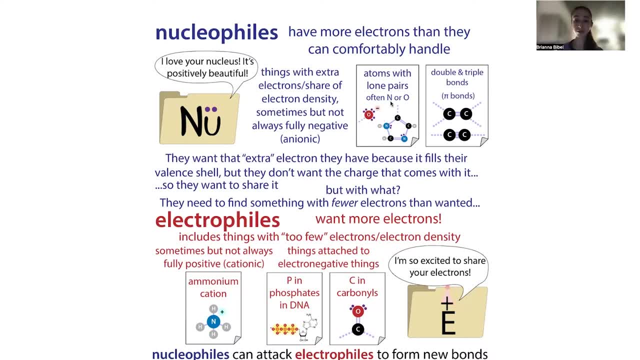 basically with a nucleophile, if you want to form a new bond, you're going to have to have the electron capacity in order to make that bond, And so these extra electrons are often coming in the form of they have a lone pair of electrons. so these unpaired electrons which you see with 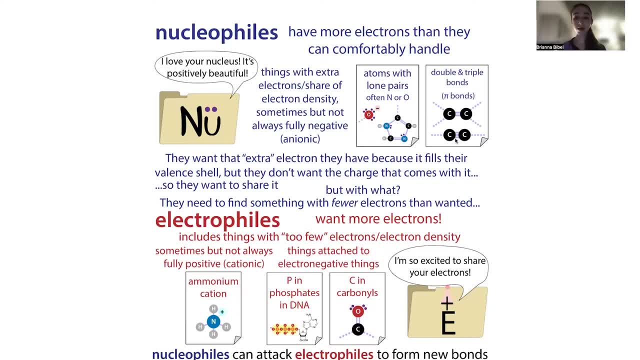 nitrogen and oxygen a lot, or you have a double bond or a triple bond. So basically there's extra electrons here that are going to be available for making a new bond, And this is what I was talking about before when you get these two dots over your U, to give you that. 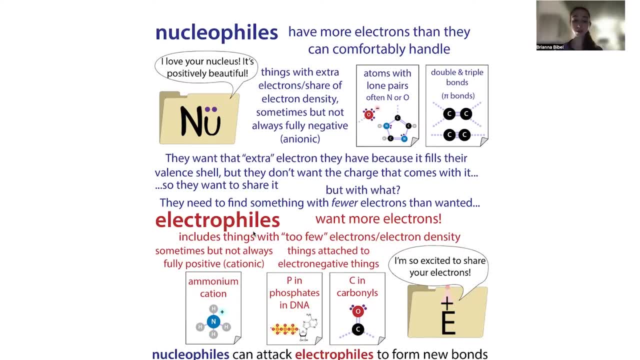 smiley face, An electrophile. this is something that's going to have less electron density than it wants, And so this is often- but not always- going to be positively charged or partially positively charged. So with positive charge you can get something like an ammonium cation. 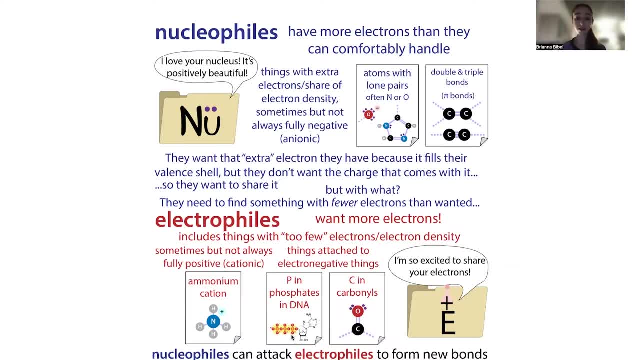 With a partial charge, you can get something like a phosphorous and a phosphate group. because you have this oxygen, The oxygen is pulling away from the phosphorous. or you can have something like the carbon in a carbonyl bond, because, again, you have the oxygen pulling away from the carbon. 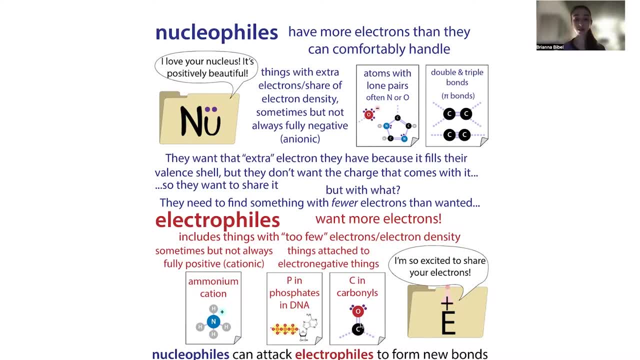 making this carbon partly positive and therefore electrophilic. So in the case of our kinase, we have our nucleophile is going to be the hydroxyl oxygen and then our electrophile is going to be the phosphorous in the phosphate group. 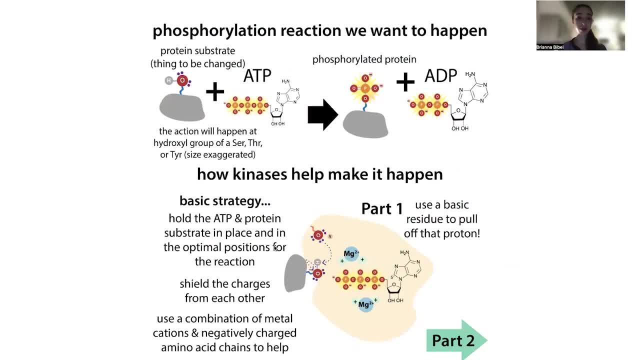 And then the, which in just the OH form. that oxygen is going to be kind of like tied up with a hydrogen, but we're not needing to have extra electrons that we can share, And so what's going to happen is the kinase is going to help deprotonate this. 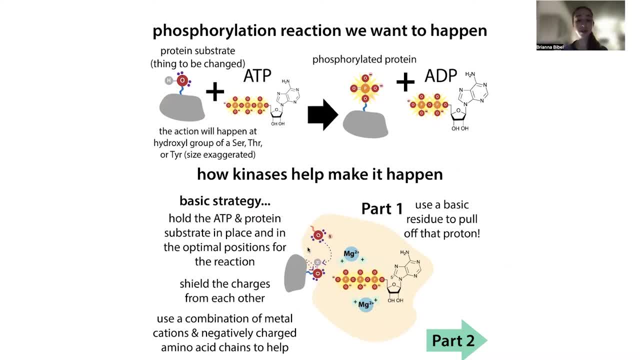 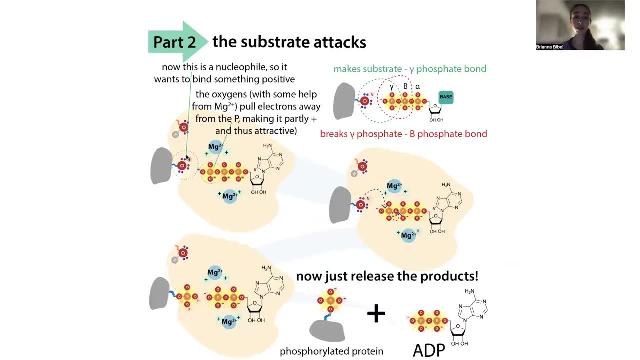 It's going to pull off that hydrogen. So now you're going to have, now you're going to have, an O minus group and this is going to be a strong nucleophile And you're going to have- remember the this negative charge is going to make this stronger nucleophile and you're going to have. 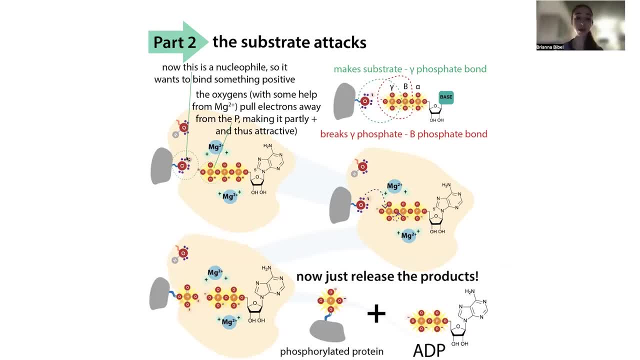 these lone pair of electrons that are going to be available in order to form a new bond. So, remember, you need a pair of electrons to form a bond. and well, here you've got an extra pair of electrons, so let's form a bond to that phosphorus, right. And then, in order to form a 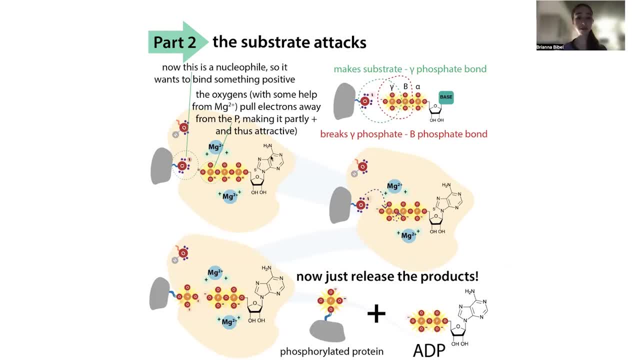 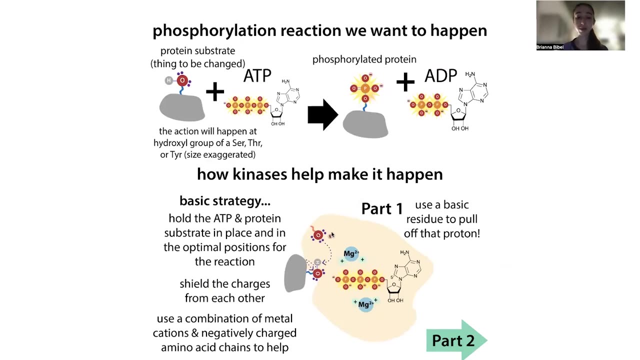 bond to that phosphorus. you're going to have to kick off the rest of this ATP and the remainder of the ATP will be ADP. so our end product is going to be ADP. So we've had the enzyme is going to be helping pull off that hydroxyl group. It's actually going to be using another oxygen in order. 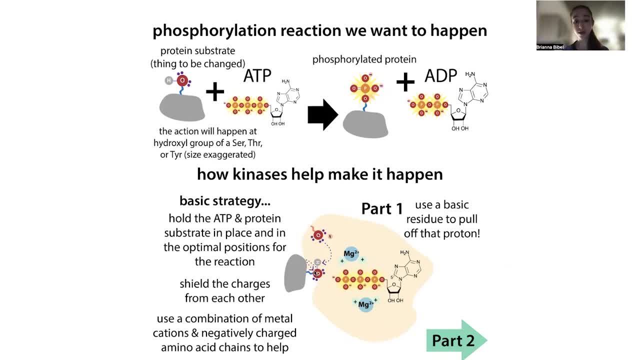 to do this. so it's going to deprotonate this hydroxyl group and at the same time, you have these magnesium ions which are positively charged, are going to be helping hold the ATP in place and making it so that things aren't repelling one another, and so this is going to help hold this. 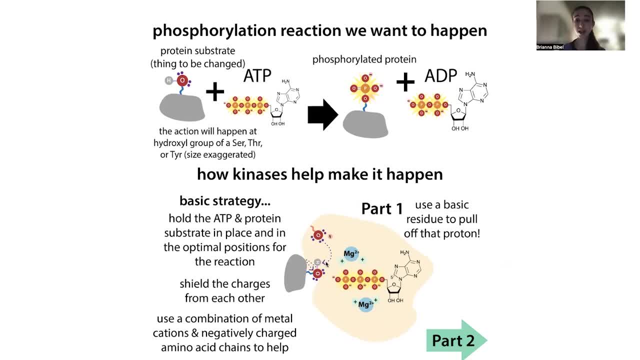 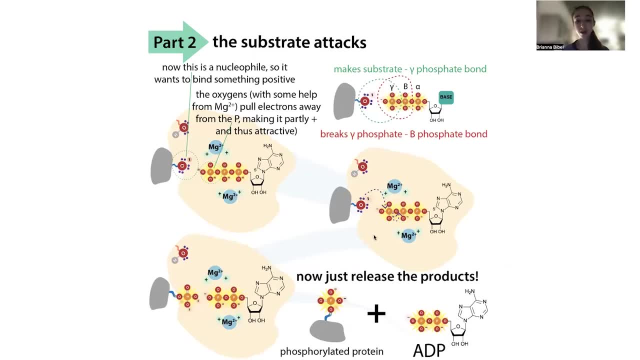 here In the position so that when this oxygen is activated, it's going to be able to attack. and so then, well, it's going to attack. So you've deprotonated this oxygen, Now it's going to attack that phosphate group. This is going to be a strong nucleophile. 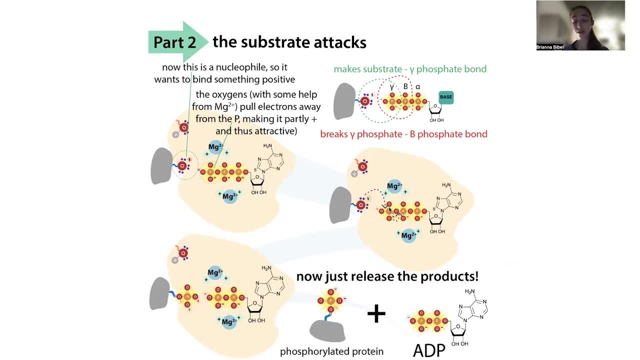 This is going to be electrophilic. You're going to get an attack on that electrophilic phosphorus. Now, when you have that attack, well, now this phosphorus is going to be attached to too many things, and so it's going to have to lose one of them, and it's going to have to lose one of them. 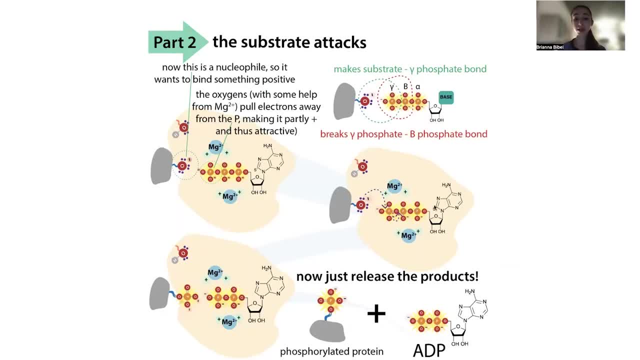 whatever was the work like a better leaving group, and so this ADP is going to be a good leaving group Basically. this is pretty stable on its own, and so it's going to get kicked off on its own, leaving your protein with this phosphoryl group attached, and so now you have. 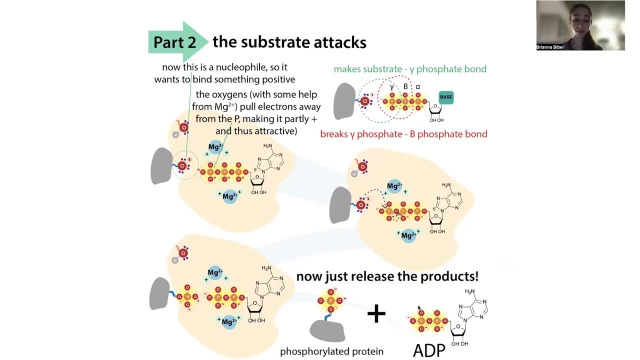 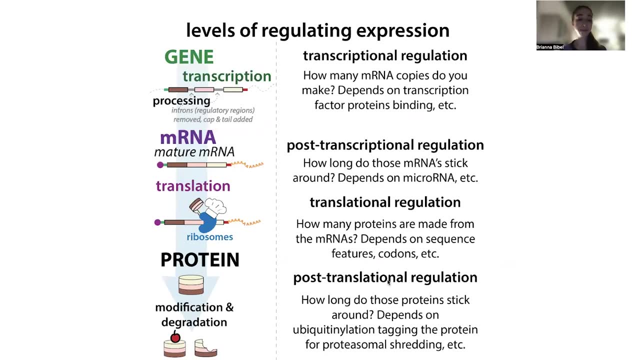 a phosphorylated protein as well as ADP, and again this is going to then dictate how the protein is functioning. It can serve as different binding sites. It can influence the protein's activity. You think of it kind of like if you pack a suitcase and then you realize you forgot something. 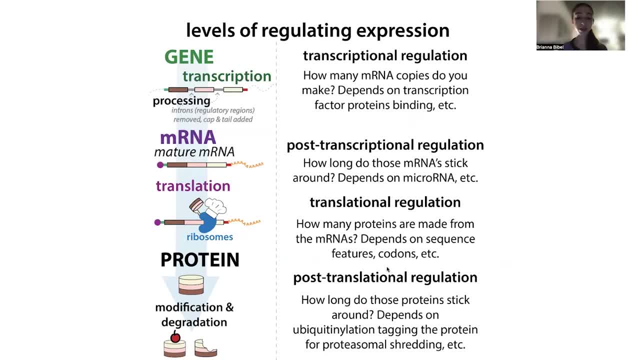 and so you add that in afterwards. If you add a big bulky thing, well now you might have to rearrange some things in your suitcase. and that's kind of what can happen in the case of a protein is you can get a kind of like shape shift, a conformational change as the protein adjusts to. 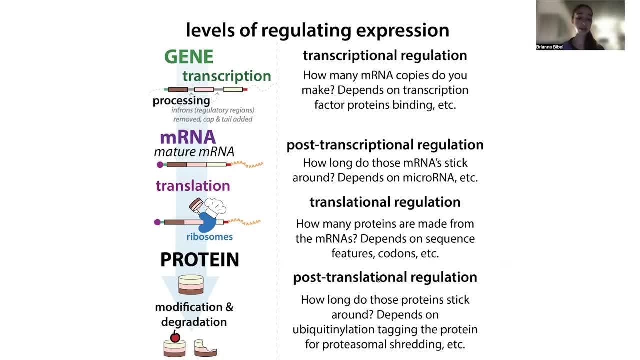 having this big bulky group on its surface and this can be a key modification that can help regulate the protein's activity. A couple more things About threonine, and then we'll do a little recap. So in terms of its metabolism, so metabolism. 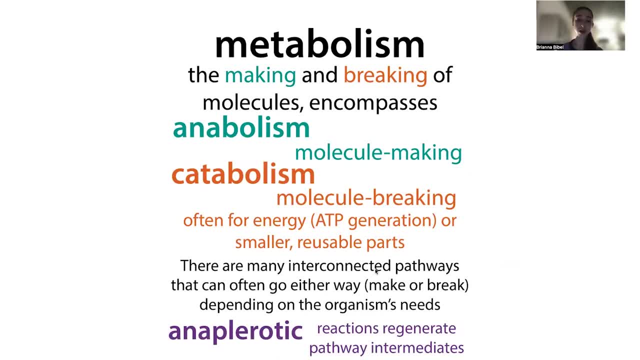 refers to the making and breaking of molecules. so we can talk about anabolism, which is making molecules, and catabolism, which is breaking down molecules. In the case of threonine, well, there's not much to say about us making them because we can't. They're called dietarily. 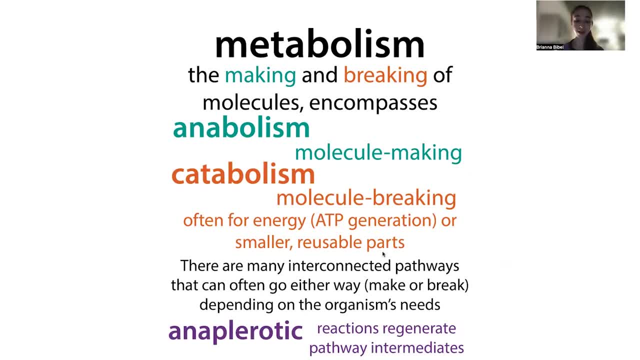 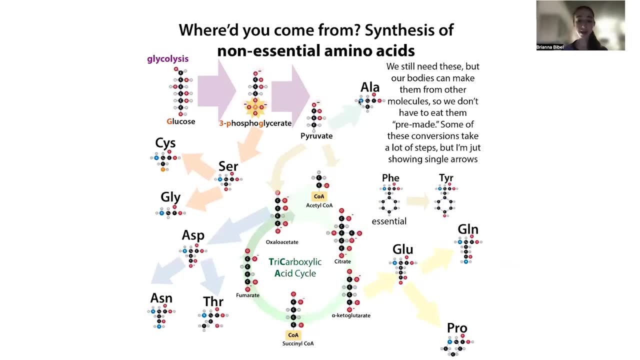 essential, which means that we need to get them through our diet. We can't get them pre-made in our food. So some of the amino acids that we would call non-acidic, which are the amino acids that are essential, we still need them, but we can make them With threonine it's going to be essential. 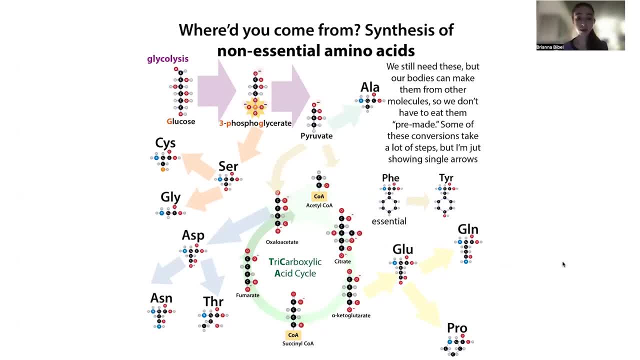 which means that we need to get it pre-made through our food. So some, like plants and microorganisms, like bacteria, are actually able to make threonine. They can convert aspartate into threonine, but our body doesn't have the enzyme, so we can't do this and it's considered as an 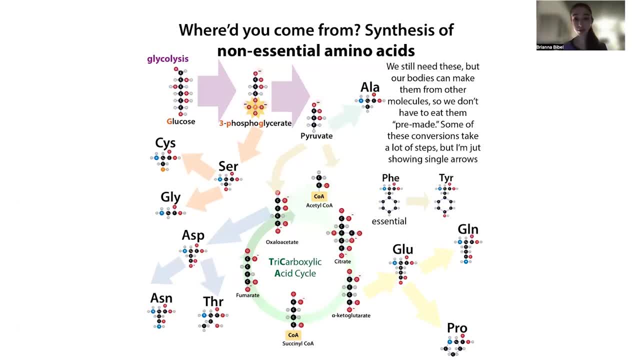 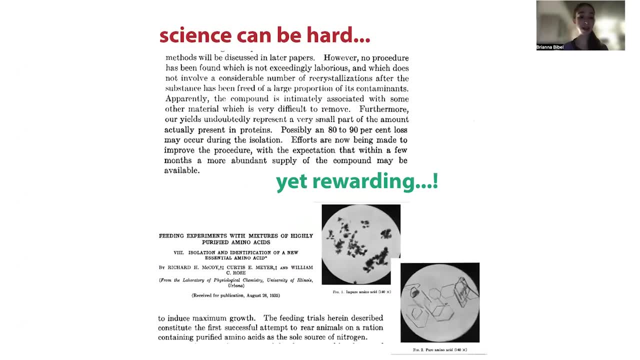 essential amino acid. So we have to get it by eating, say, those plants that were able to make it And how. this is essential. this was figured out. This was done by a scientist named William Rose and with the help of some grad. 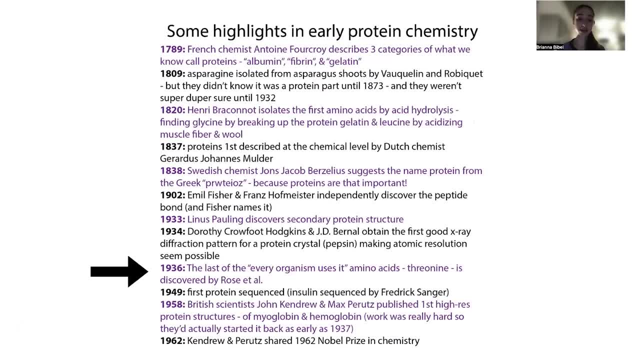 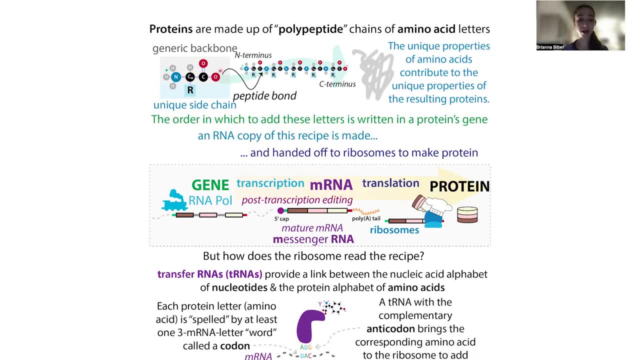 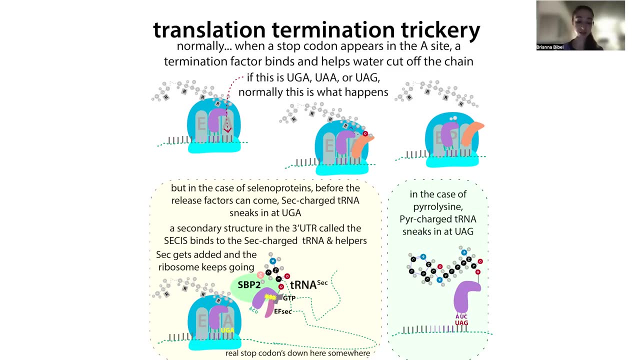 students. And so, basically, threonine was the last amino acid to be discovered, at least the last of the 20 genetically common, genetically encoded ones, so the ones that our body uses most in our proteins. And there are a couple of extras that we'll talk about, like selenocysteine, which is a 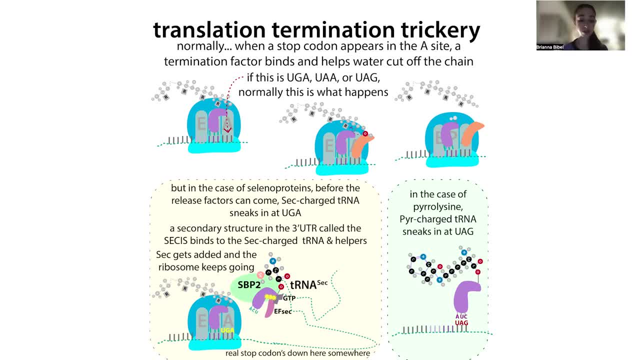 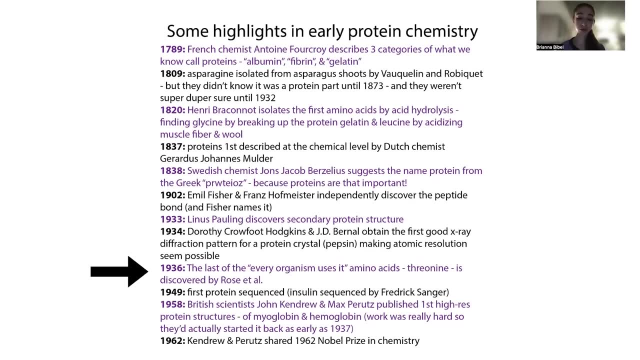 special case, as well as pyrolysin, which is used by bacteria. But for the most part we have a core set of 20 amino acids And then we get that further variety by adding on things such as phosphorylation through these post-translational 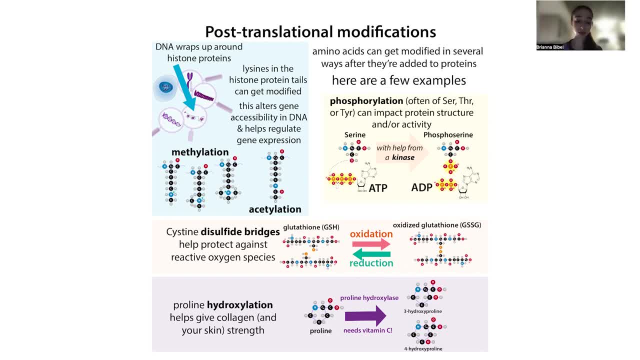 modifications. And remember that can only happen if you have some sort of functional group that's going to allow it to happen. So if you don't have just like a pure hydrocarbon where everything looks the same, but if you have something like a hydroxyl group where now you have something, 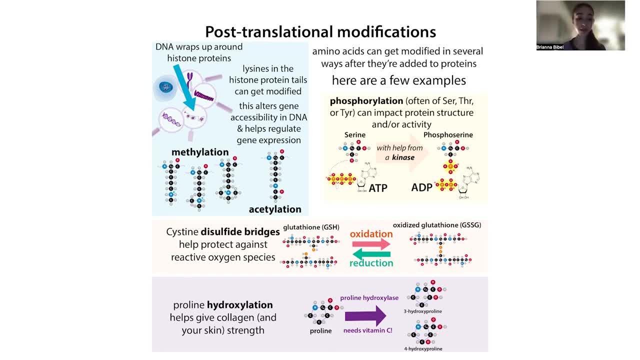 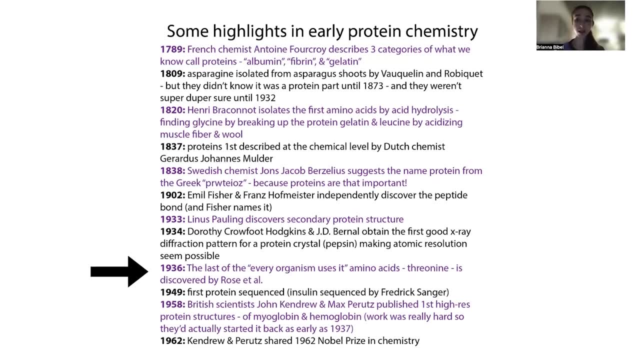 more reactive, then you can get these modifications. So we have a lot of different types of amino acids, such as phosphorylation. But going back to the concepts of threonine, it was the last of these 20 common genetically encoded amino acids. 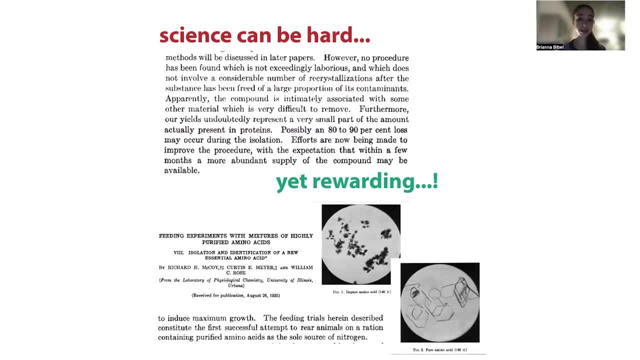 And it was discovered in 1936. So basically, in the 1930s, William Rose was trying to figure out: okay, well, what are the essential amino acids? What amino acids do animals need in order to survive? And so he started with working with rats And he was taking what was known about the. 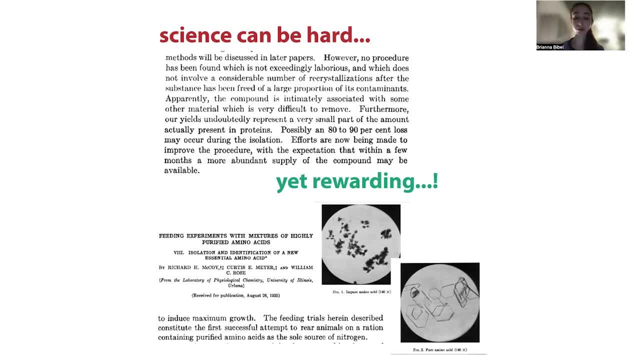 amino acid, the essential amino acid- And he was taking what was known about the amino acid- essential amino acids- and feeding them to these rats, and the rats weren't surviving. so there was something missing, and so he wanted to try to figure out what that missing thing was. so we took a bunch. 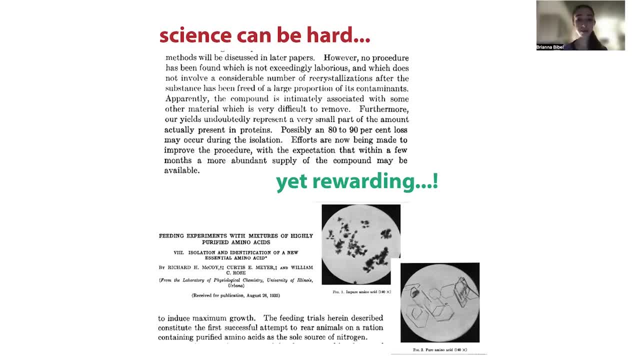 of protein and he tried to separate out its different components, isolate all of the different amino acids and add them to that mixture of, to the mixture of known components, in order to see what would allow the rats to survive and thrive when he added it. now, this was a very grueling. 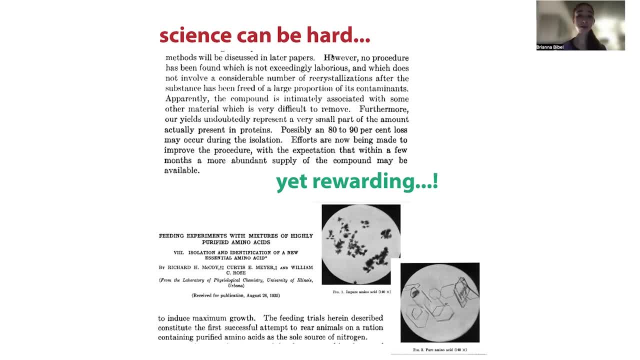 process. as you can tell from his paper, however, no procedure has been found which is not exceedingly laborious and which does not involve a considerable number of recrystallizations after the substance has been freed of a large proportion of contaminants. blah, blah, blah. possibly an 80 to 90. 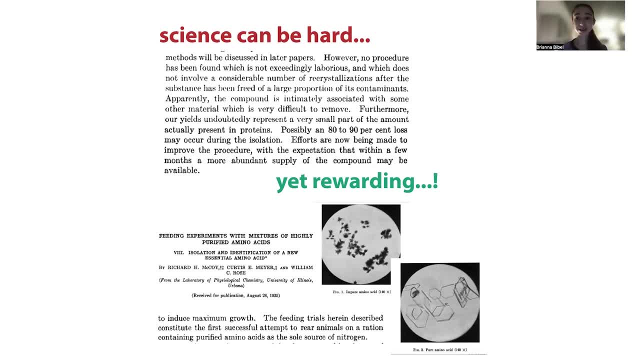 percent loss may occur during isolation. yeah, so basically it was a lot of hard work, but at the end of the day, he was able to discover threonine and then to show that it was that it was essential. you actually, in addition to feeding rats and dogs, he enlisted the help of some grad student volunteers. 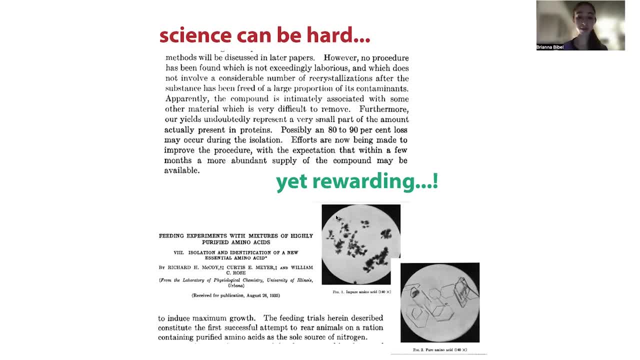 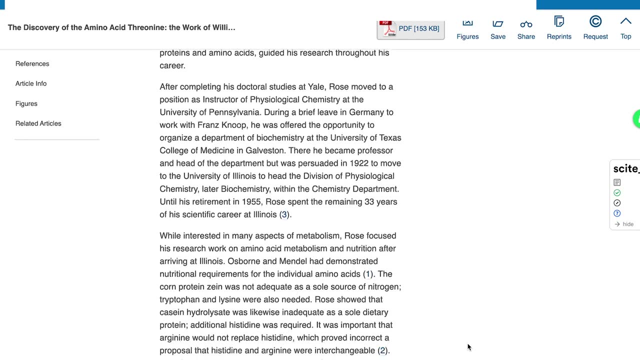 who ate a defined diet which contained this threonine, and he was able to show that they got grumpy and stuff and that they needed this threonine in order to survive, and so i will link to a cool article describing these recent experiments in this classic paper, which is: 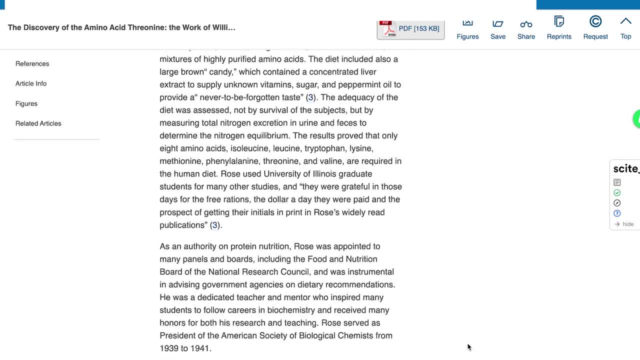 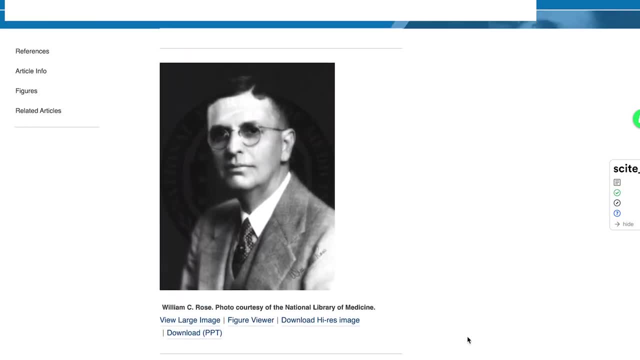 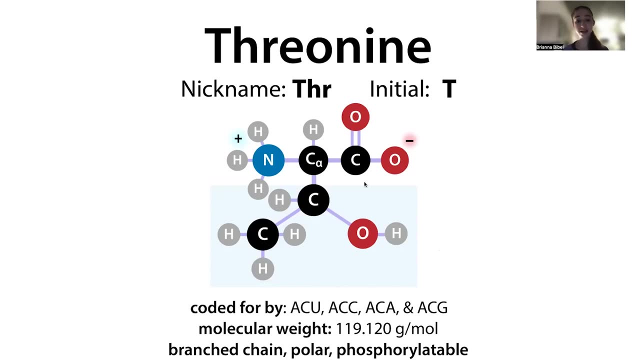 pretty interesting, but threonine was the last of these amino acids to be discovered, but, as we'll talk about later, we also have some, some cool exceptions to the rules and things like that. so, to review, this is threonine, um? it's abbreviated thr or t. it has these three groups. 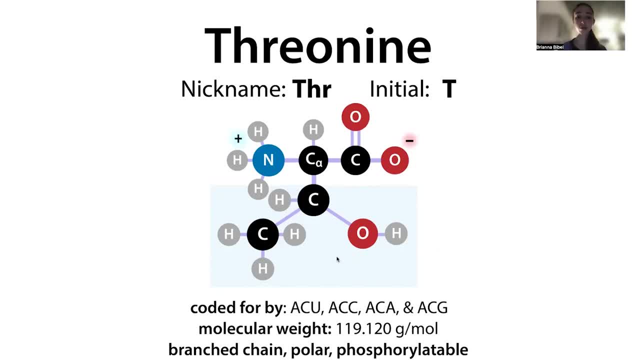 you can remember um. so it has these three groups in its side chain. one of them is an o, so three o mean um. that's not really how it got its name. it has to do with it having a similarity to the sugar threonine. but um, if that helps you remember threonine, there you go. 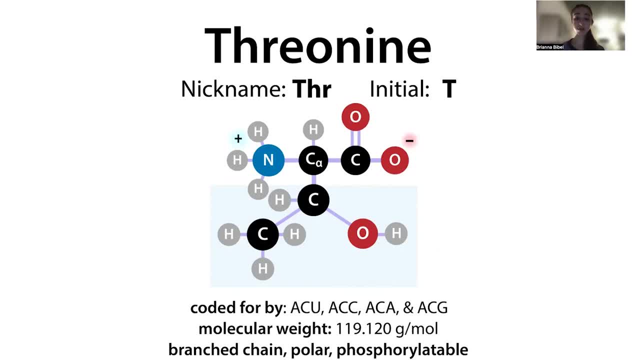 what else to remember about it is that it's going to be polar and it's going to be phosphorylateable. so it's polar because it has this oh group. this oxygen is going to be electronegative. it's going to pull the shared electrons away from the 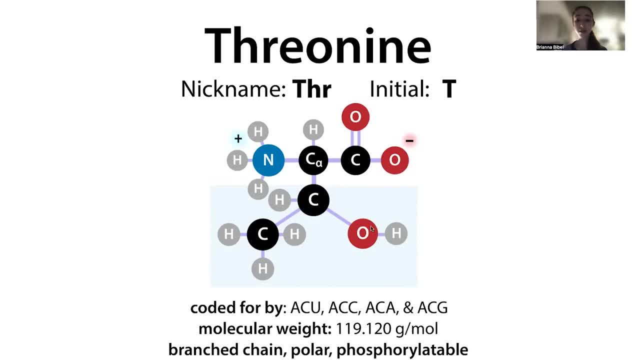 hydrogen and away from the carbon. it's going to make this partially negative, other things partially positive. it's also going to make the oxygen nucleophilic. so it's going to be seeking out something to share all that negativity with. it's going to be sharing, seeking out a lot of. 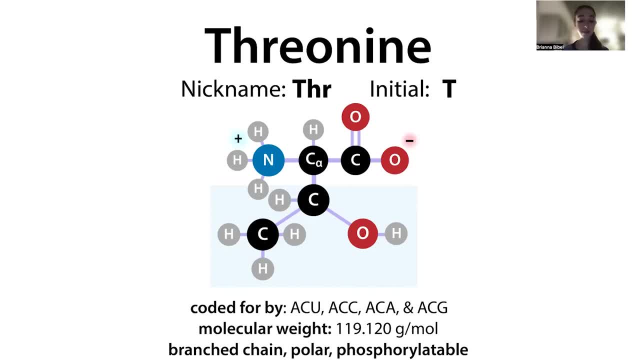 electrophile, such as the phosphorus in a phosphate group of ATP. This is going to allow it to get modified post-translationally, such as through phosphorylation. When you phosphorylate a protein, this can influence how the protein is going to act and can change the protein shape and things. 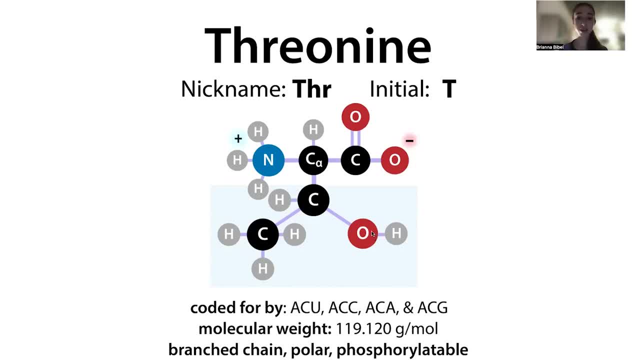 like this. All of this is happening because the oxygen is kind of opening up opportunities for modifications, for reactions, because this oxygen is going to be kind of more interesting than when you have a pure hydrocarbon, when you just have carbohydrates and hydrogens. 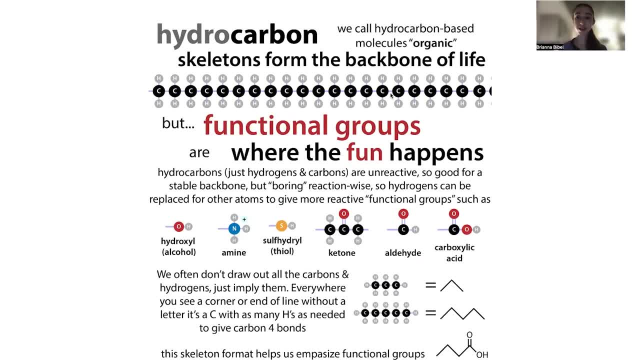 Here there's nothing really interesting. There's nothing interesting for water to hang out with. so water would cause this to be hydrophobic, so water would exclude it. But when you have some liquid oxygen now you have a partial charge. Well, water is going to be cool hanging out with. 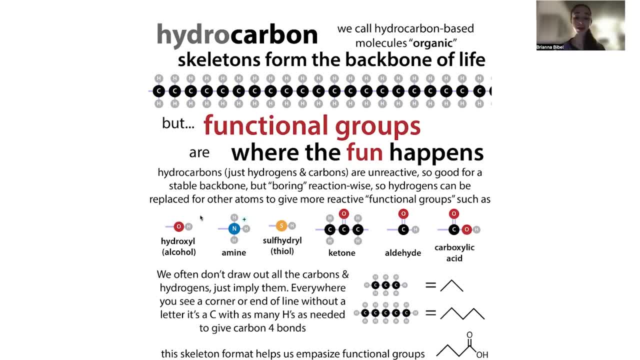 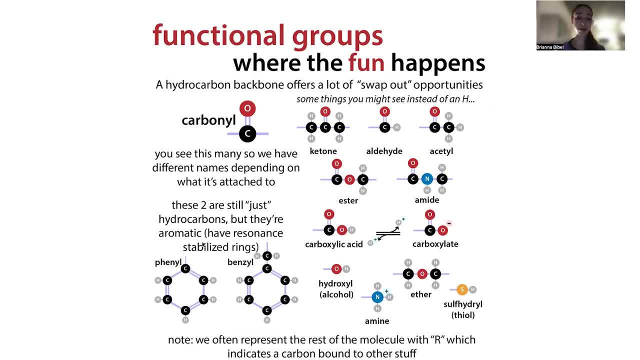 that. so you have more hydrophilicity And, additionally, you're going to have a kind of functional group. You're going to have something on the molecule where reactions can happen. Now you have a place that is vulnerable to attack. You have a place that can attack. You have a place where there's something for an enzyme or another. 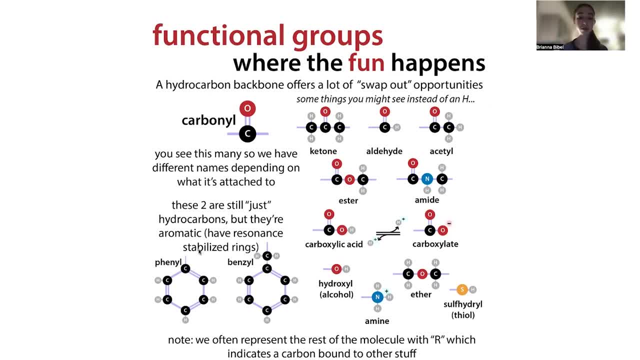 molecule to bind to. There's basically something different that's going to make it unique from the surrounding hydrocarbon skeleton And when you have one of those unique spots, you have the opportunity for reactions to happen, for binding to happen. You have the opportunity for diversity to happen, for these molecules to do things. 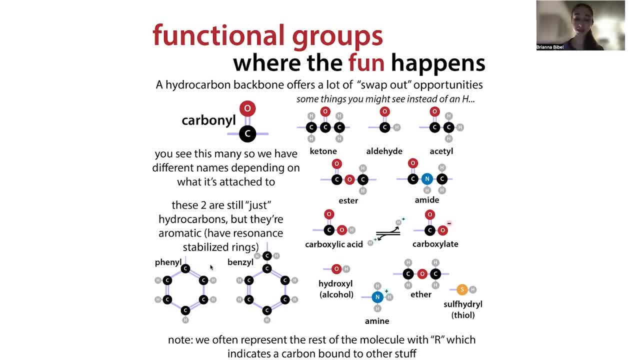 to be different from one another, And so this is just the first example of a functional group we're going to look at. This hydroxyl or alcohol group is going to be a really core one, And you're going to find it in the amino acids. tyrosine, serine and threonine is where you're going to find this OHR. 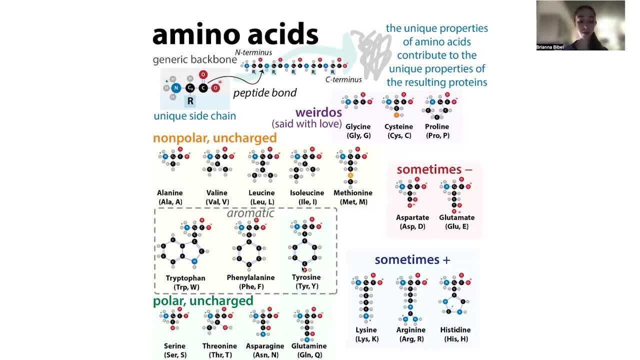 this hydroxyl group, And so all three of these are going to be capable of being phosphorylated. They get phosphorylated with the help of enzymes called protein kinases, Serine and threonine. these are often phosphorylated by the same kinase.